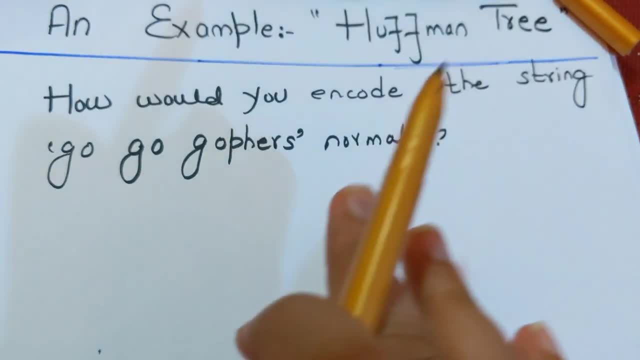 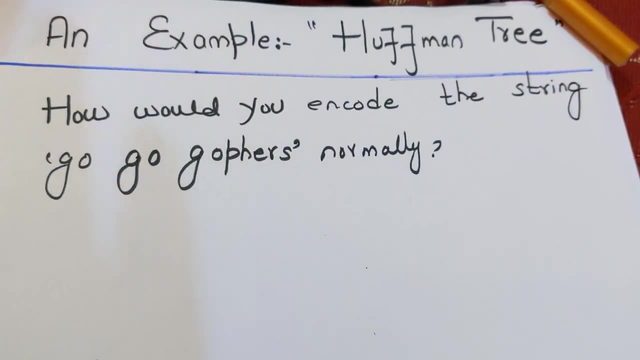 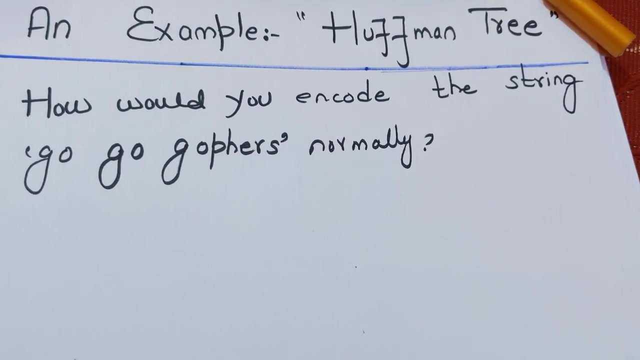 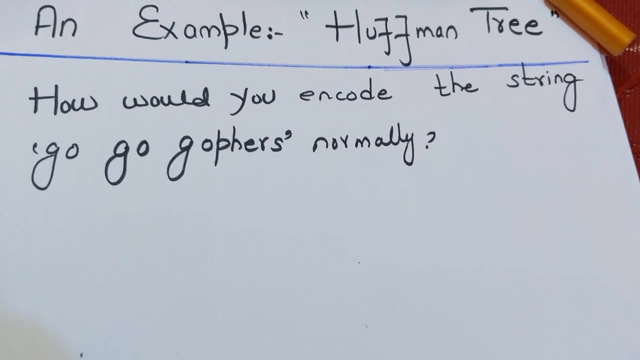 With the help of this algorithm, you can easily compress your information without losing any data. That's why we can say it is losslessly Huffman coding algorithm. Okay, That's why we can say it is lossless data compressing algorithm. It is most widely used in alpha numeric data. In Huffman tree, we applied the approach of bottom up approach. Okay, What is bottom up approach? Like this Bottom up approach may apne. 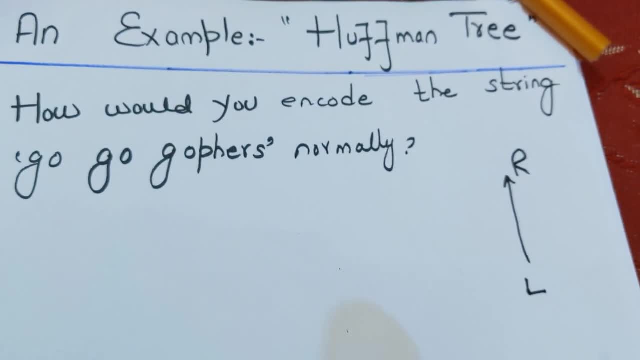 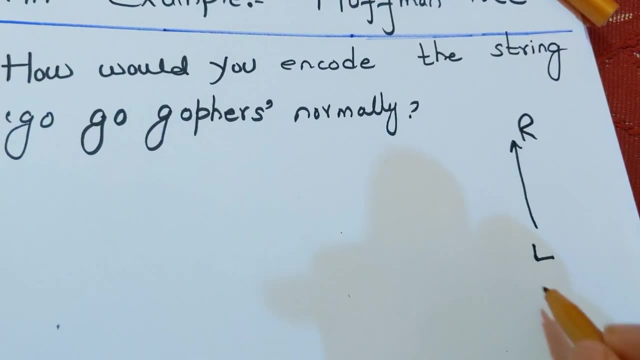 leaf se jaana hai root tak. But in the top down approach, the first approach is bottom up and the second approach is top down. We are applying in Huffman tree. what bottom up approach. This is bottom up, Okay, But in the top down approach, like binary tree, you have to move. 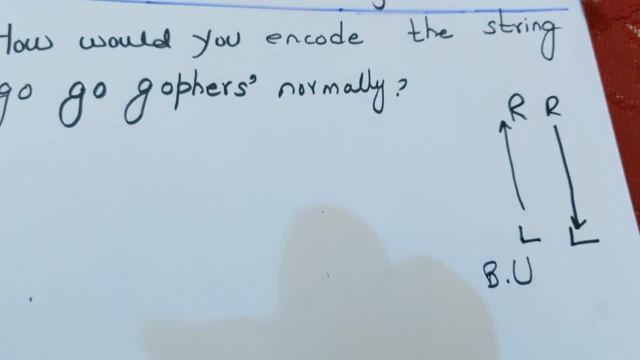 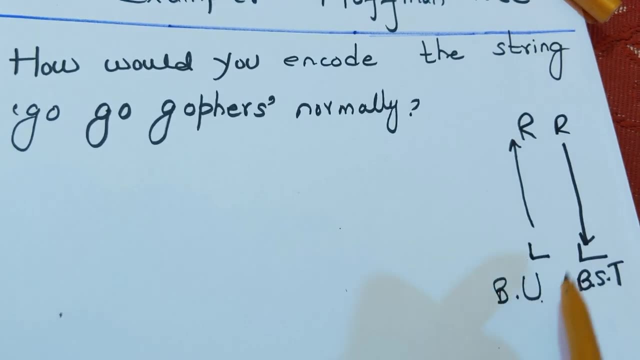 forward from root to leaf. Thike Ye apki hai binary such tree ke approach. But in the huffman tree you have to apply bottom up approach. But in the binary such tree you can applyatalumb treeu b sakte top-down, Which is the one axis arrow gives horizontal spicy. 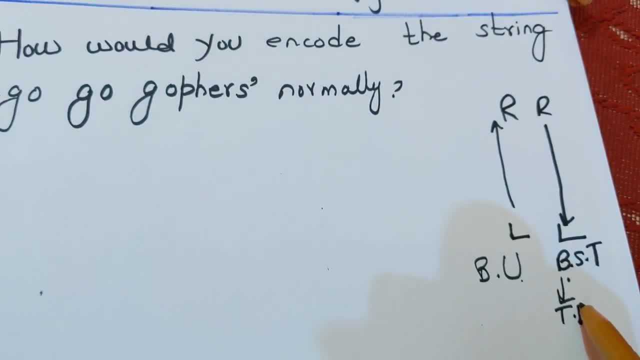 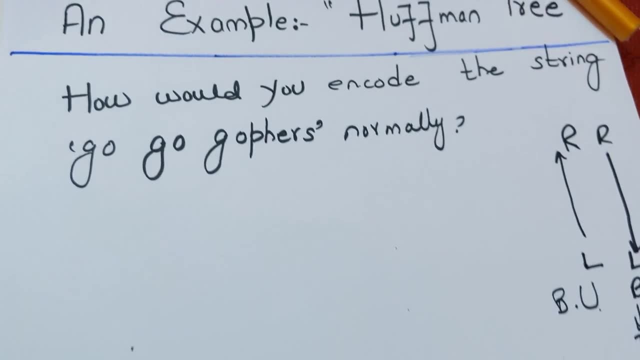 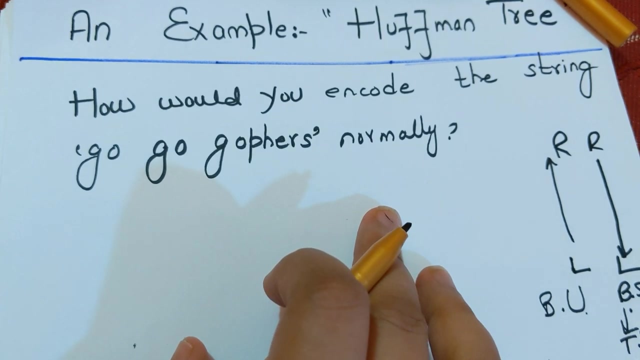 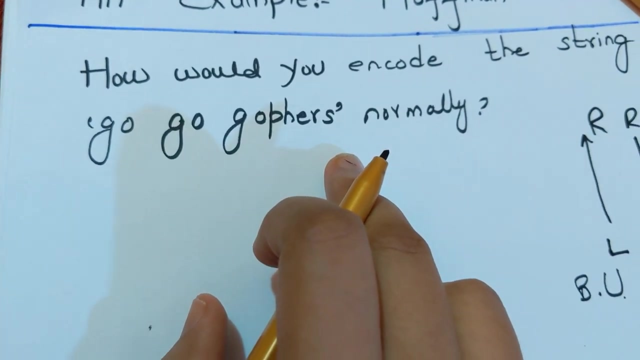 top-down approach, top-down, anyways, start. let's design it. so what you have string is go, go, go, for what you have to do is encode it. so go, go, go. for if you want to encode, then what you have to write first, you have to write its binary, sorry, its. 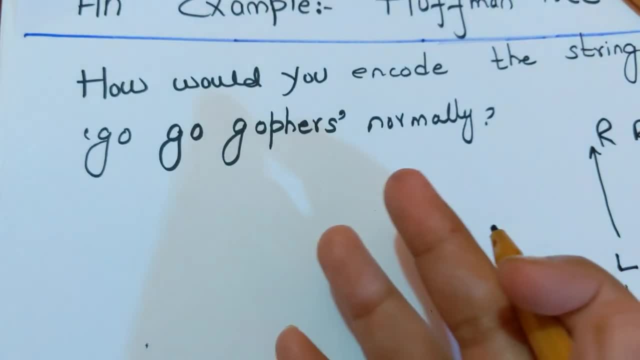 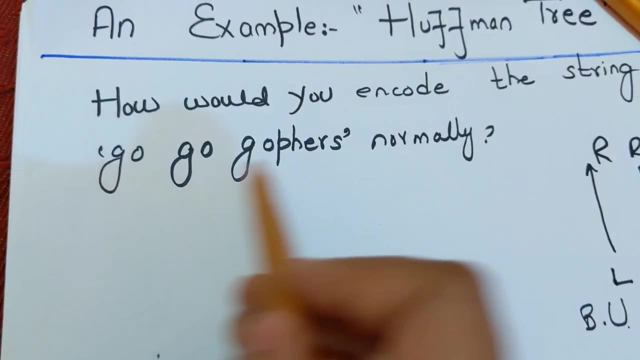 you have to write its ASCII. ok means, behind every character there is ASCII. computer understands ASCII. so G has different ASCII, O has different ASCII and all are small letters. so what is the ASCII of all? it will be in small means, it will be ASCII of small letter. so if I 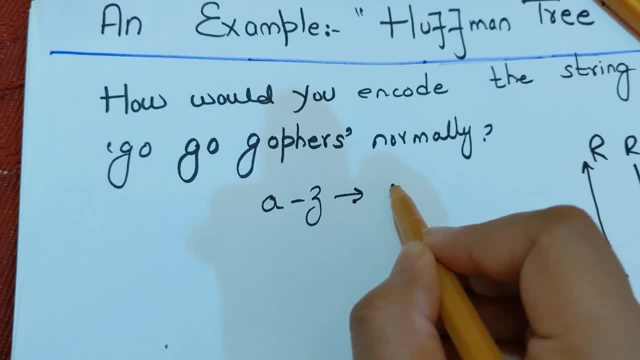 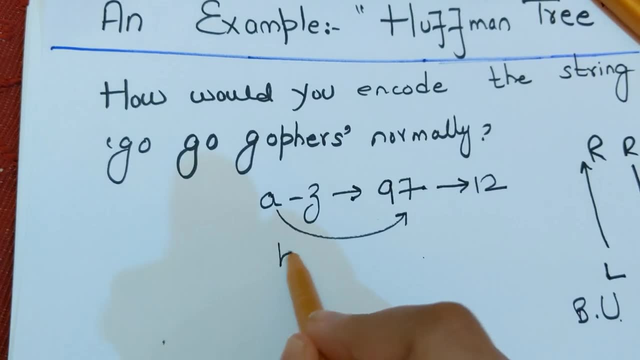 tell you that. what is the ASCII of small a and what is the ASCII of small z? small a is 97 and small z is 122. that's mean what is the ASCII of small a 97? what will be the ASCII of small b 98? 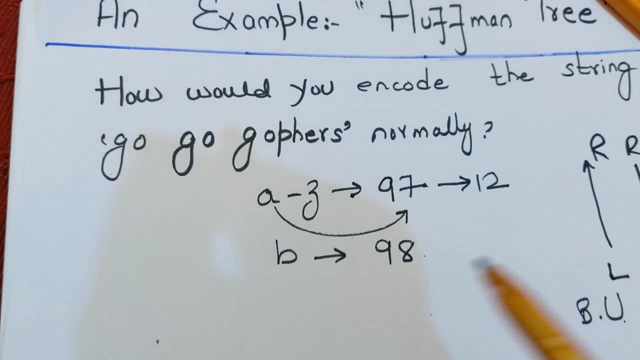 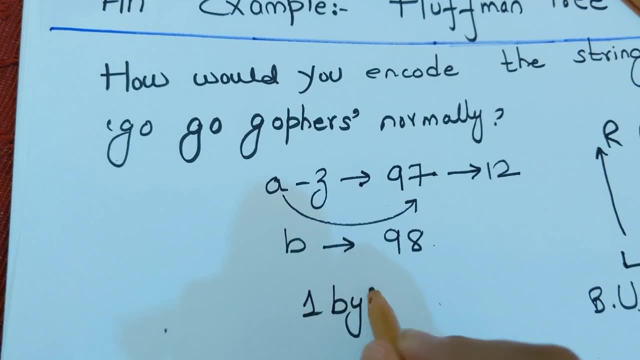 in this way, what you have to write for every character is ASCII. after writing ASCII, you have to write ASCII of all characters. you have to write ASCII of all characters in 8, 8 bits, because you know one byte is equal to 8 bits. one byte is: 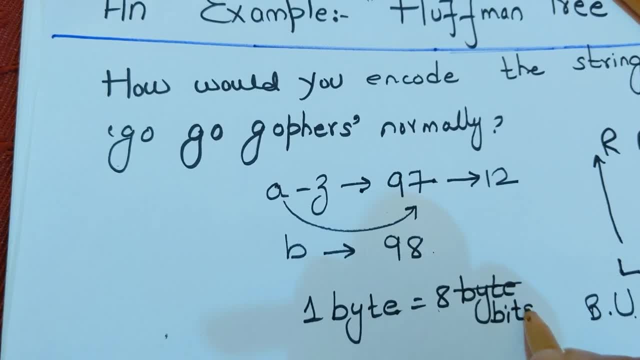 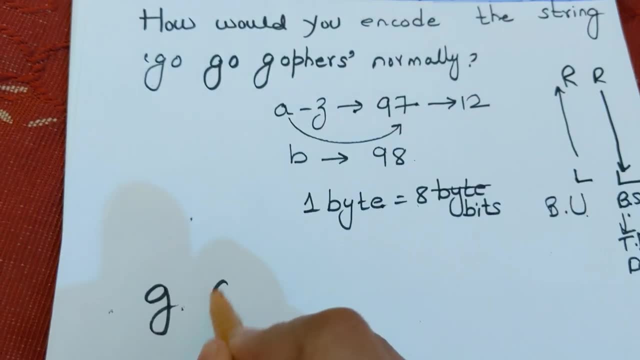 equal to 8 bits, sorry, 8 bits. so that means on every character you have 8, 8 bits of hide. so first of all, what do I write? I write its ASCII, what is the ASCII of G? then I will write again G, then again O, then the whole word. 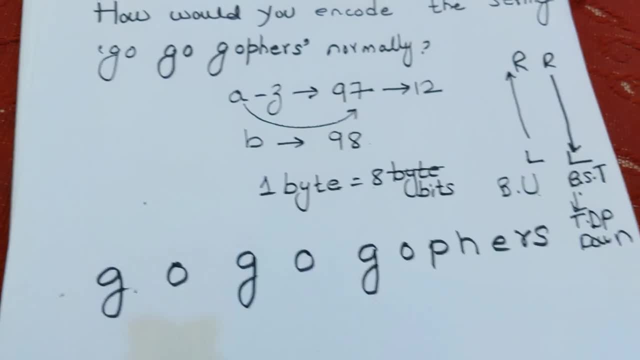 G O P H E R S. so I am going to write ASCII of all. now, here you will see when you are going to write G's ASCII. here you will see when you are going to write G's ASCII. so what is the ASCII of G? G's ASCII is 103. 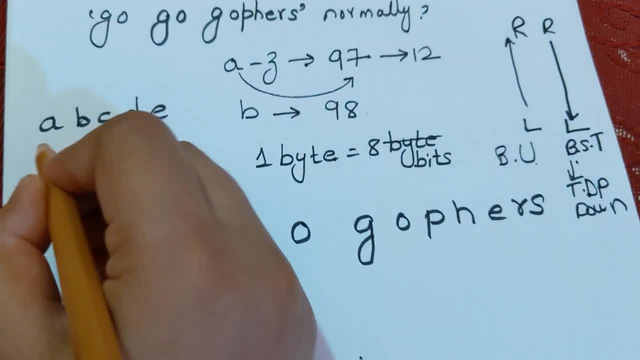 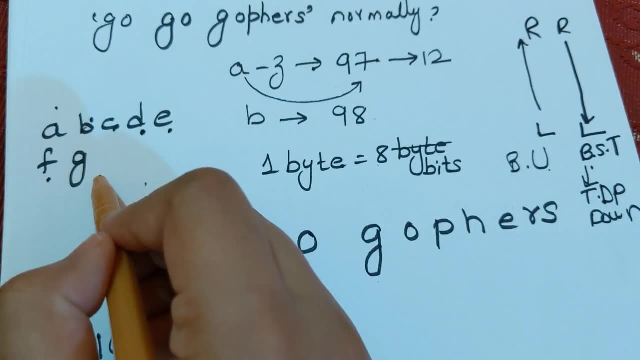 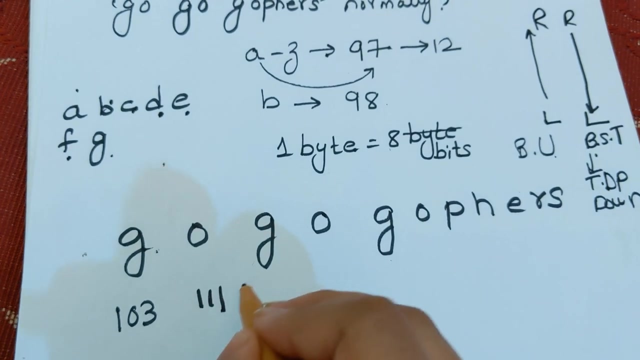 how: A, B, C, D, E, F, G. so this is 97,, 98,, 99,, 100, 101,, 102 and then 103,. in this way I will write all the ASCII of all characters here. 103 is O, then that's mean 1, 1, 1, 1, 32. 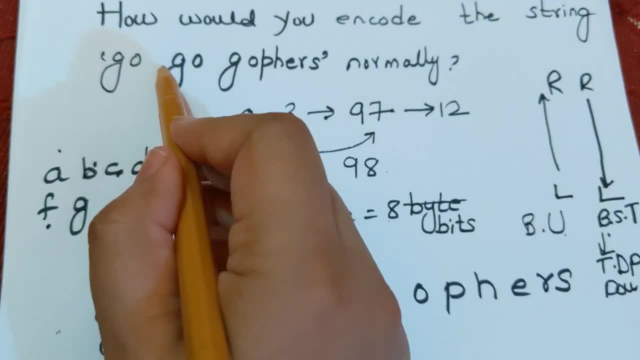 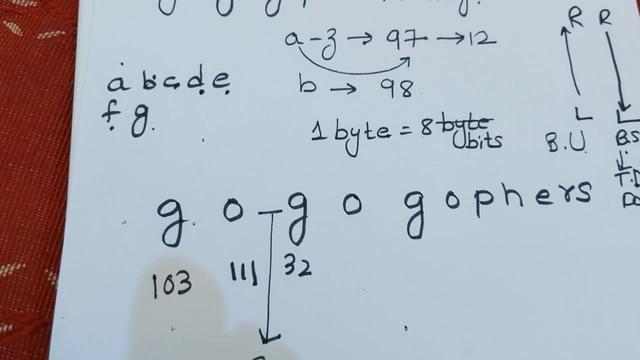 note one thing: after GO, you have space here in computer. space also has ASCII. So after this go, what is your space? And do you know what is the space of this? Its Q is 32.. So instead of writing here, I have written 32 here. 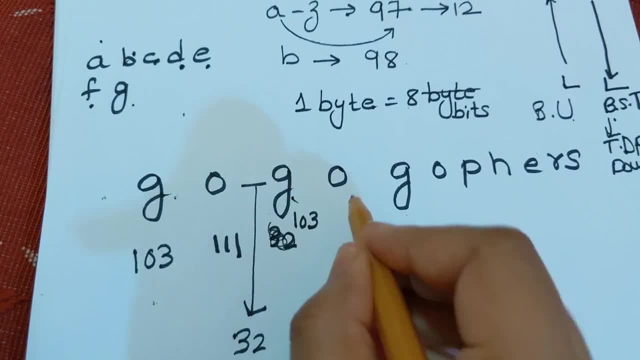 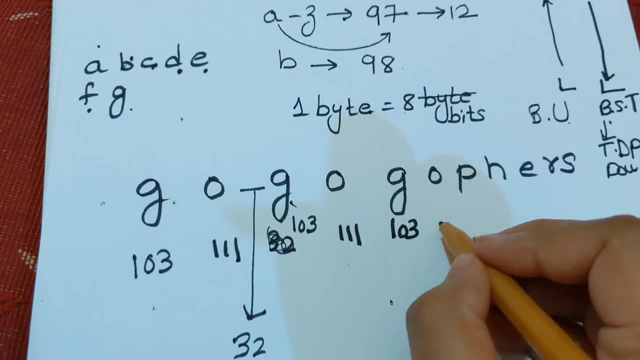 Again G is repeated. That means again your ask is 103.. Again your O is repeated, so 111.. Again G is repeated, so that means 103.. O again is repeated, so 111.. So I have taken the string in such a way that it comes in repetition and I don't have to take out more ask. 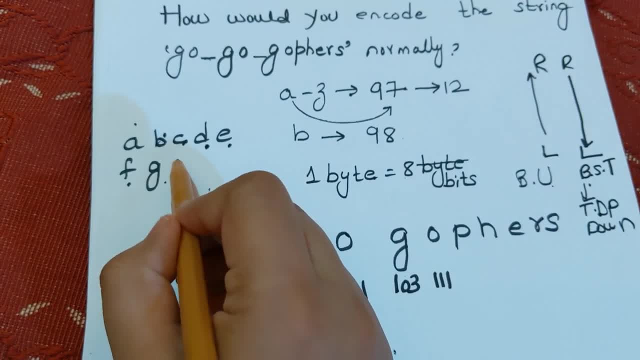 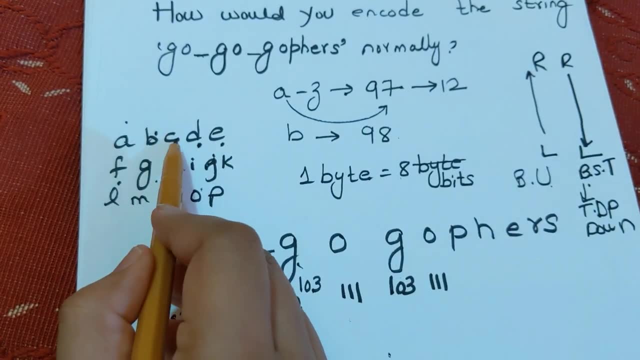 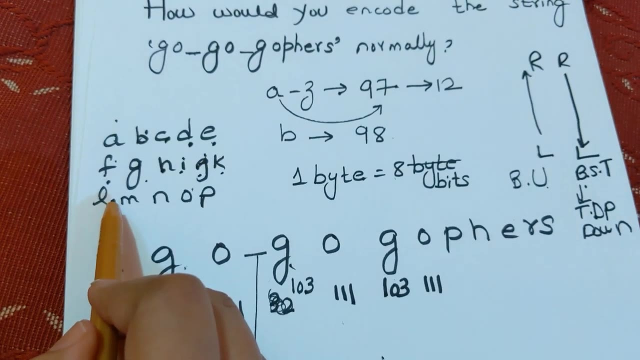 P is there, So P's ask will be A, B, C, D, E, F, G, H, I, I, J, K, L, M, N, O, P. Now calculate 97, 98, 99,, 100,, 101, 102, 103, 104, 105, 106, 107, 108, 109,, 110,, 111, 111.. 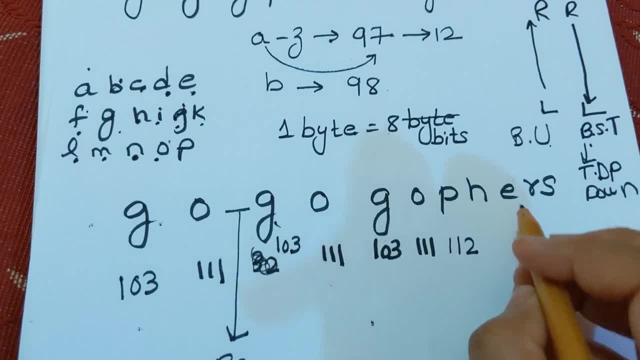 I have written it correctly here In this way. I have taken out P, 112, H. I think 104 only, I think not. I am sure 104 only will be made. If I take out E, then E will be made. 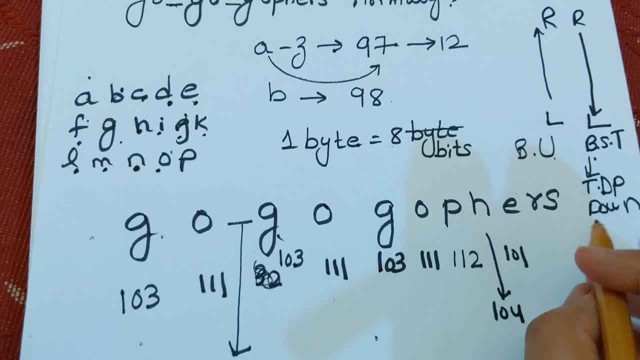 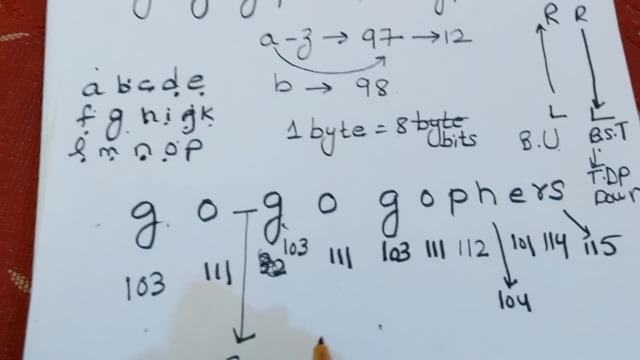 You have 101.. If I take out R, small R, then I think 114.. Diamond sure is 114 only And ask's ask is 115.. Okay, So now I am converting your data, your string, without half-mentory. 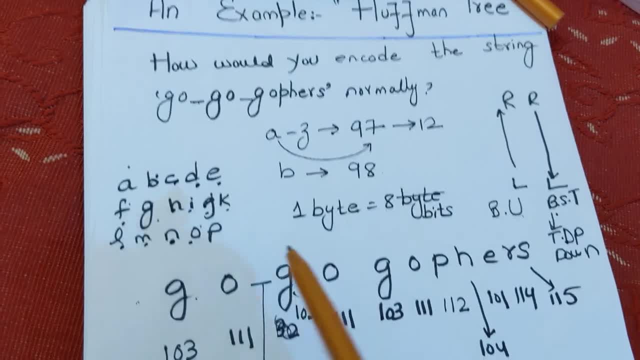 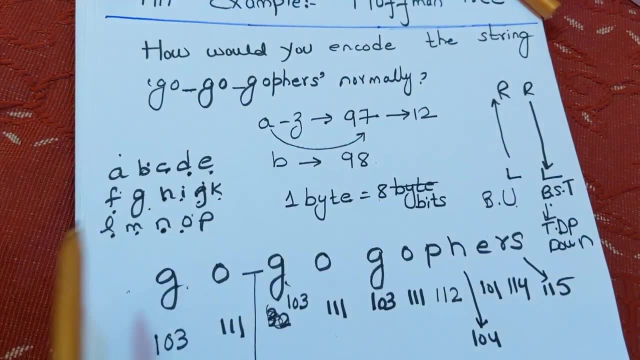 Normally, as I have written. normally, I am converting it to encode. I am encoding your information. What is encode? Go, go go first. What is the string for encoding: Go, go, go first? So what I have done in the first step is: I have written its ask. 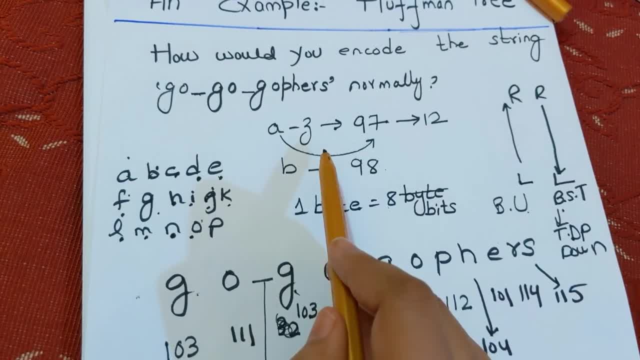 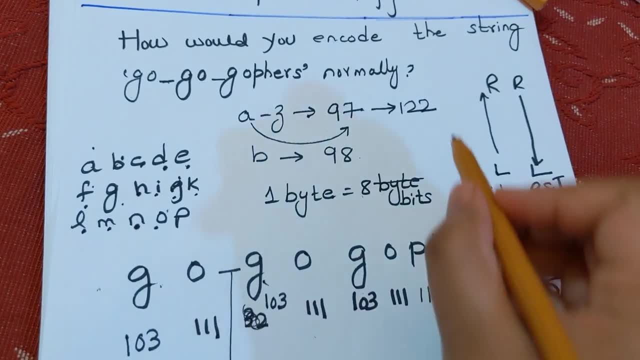 I know how to write, ask: The small a is 97.. What is the small z, 90,? sorry, it is 122.. I have written it wrong. It is up to 122.. Okay, If I talk about capital A to Z, I will tell you, just for the knowledge. 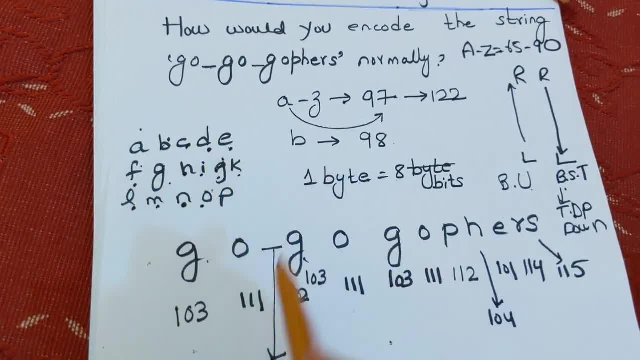 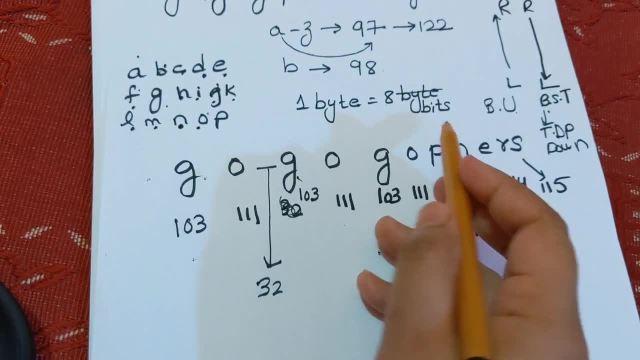 So 65 is up to 90. So here we have written the ask behind every character. After writing ask, now you have to convert every character into binary And you have to write its added bits. What do you have to do? You have to write, that is how many bits are behind every character. 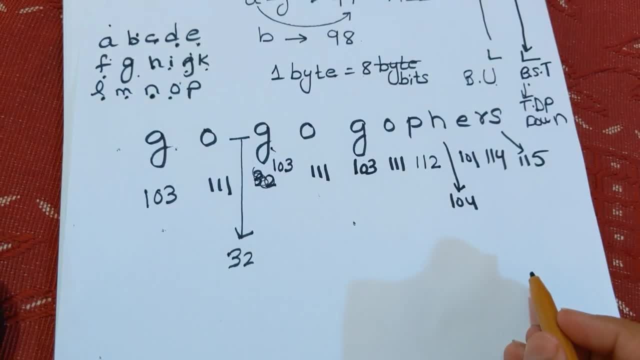 Added. So how do you normally write a binary? How do you write it? Either you make a table or you divide it From 1,, 0,, 3 to 2,, 2,, 5,, 10, and then so on. 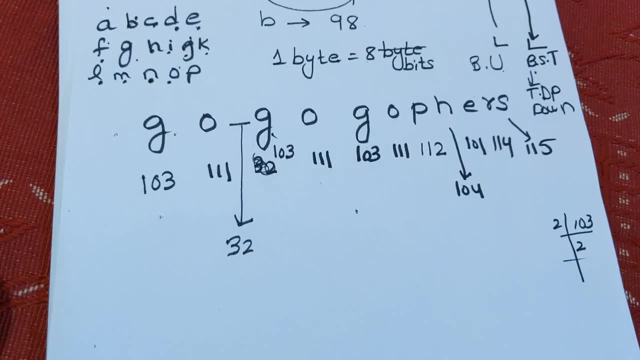 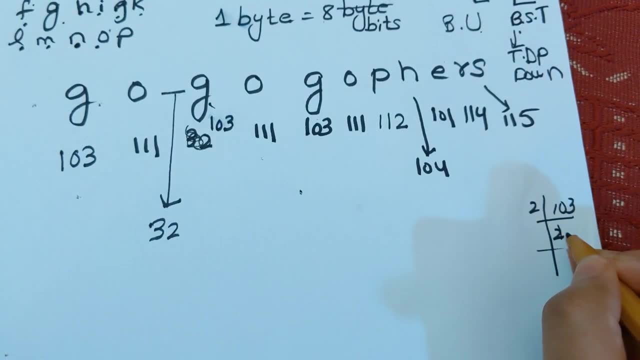 Your binary will keep on going. What you have to write in this way is you have to write binary. So to write binary, let's start First of all. let's write the binary of G. So you make a table. take LCM: 2, 5, 10, 2, 1, 2.. 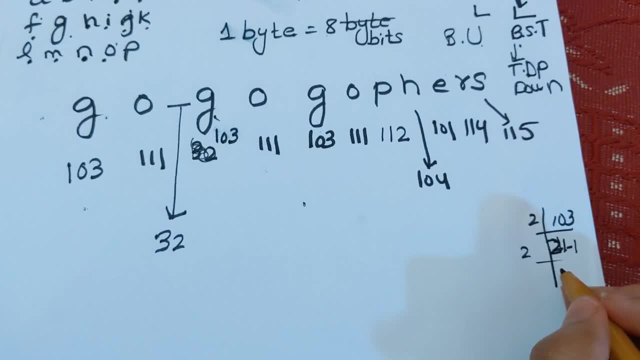 2, 5, 10, 2, 1, 2,, that is 2 out of 3, 1 is left. 2, 1, 2,. okay, now what happened? it was 2, 5, 10.. 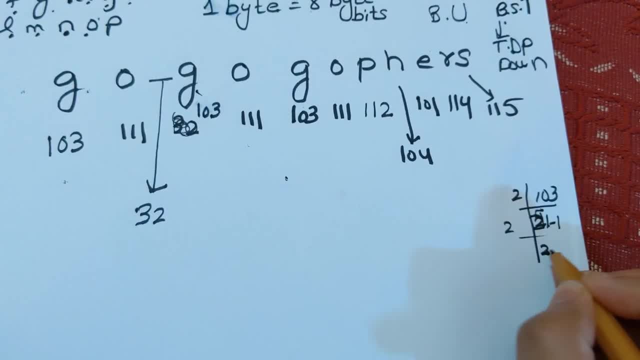 Now it is 5, 1, sorry, okay, it is 5, 1.. 2,, 2,, 4. And then 2, 5,, 10, what is left Then? 1. 2,, 1,, 2.. 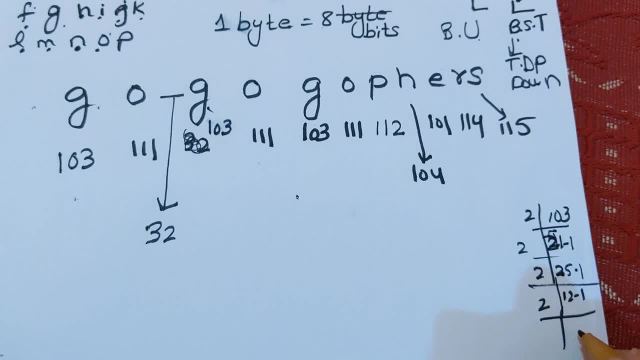 2, 2, 4,, then 1 is left, 2, 6, 12, 0 is left, 2, 3, 6, 0 is left: 2, 1, 2, 1, so you should know this. 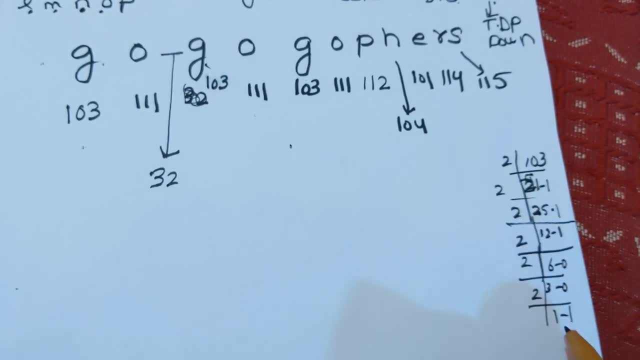 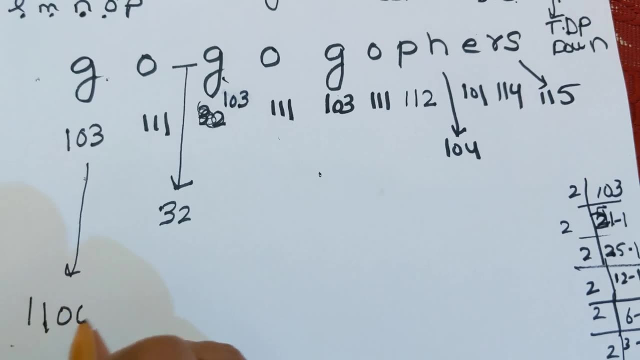 Now you write: what is your triple 1,? double 0,, 1, 1?. What is it? What is it Triple 1,? on this side you have double 1,, double 0,, triple 1.. 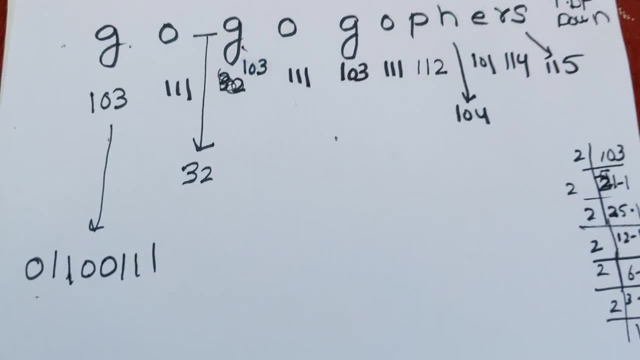 So how many are there? 3,, 4,, 5,, 6,, 7,, 1,, 0,. you write it yourself. How many are there? 8.. So in this way you have taken out O. As I know, O is triple 1.. 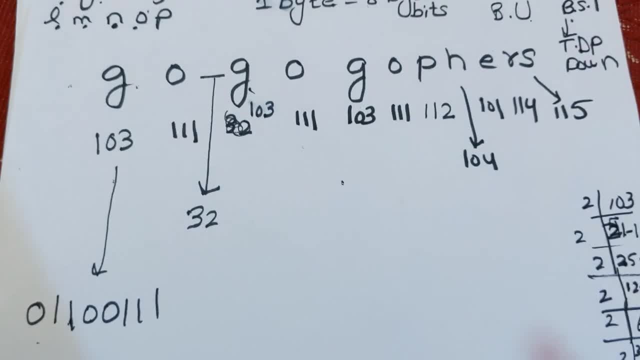 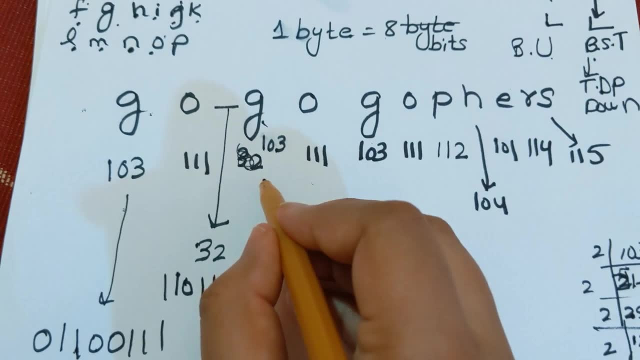 When I divide it from 2,, what will be its binary. So I am writing here what will be O's binary: 1, 0, 1, 1, 0, triple 1.. Okay, What will be G's binary? 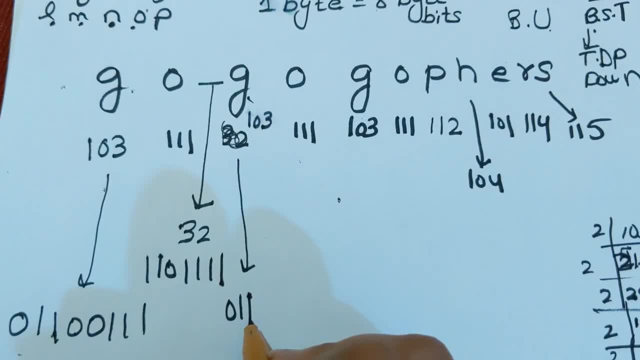 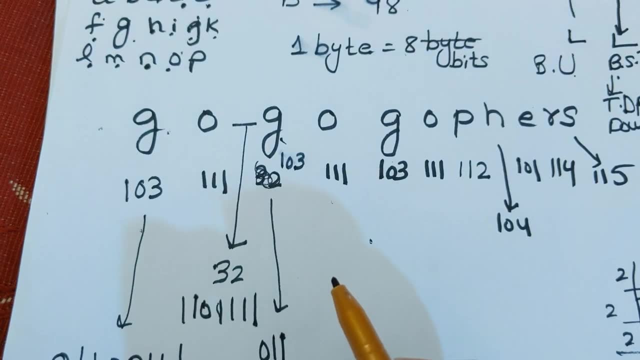 It will be the same. So 0,, 1,, 1.. Okay, after this I have to write the binary of space. So what will be the binary of space? I will do the binary of space like this: This is your O's binary. 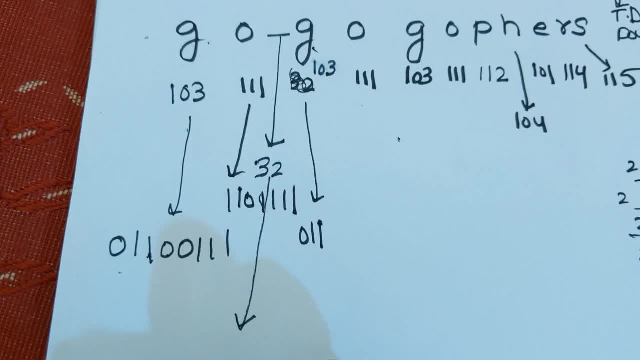 Okay, Okay, I will write the binary of space here. What will be the binary of space? Your space is 32, so the binary of space will be your double 1, 1,, 2,, 3,, 4, 5.. 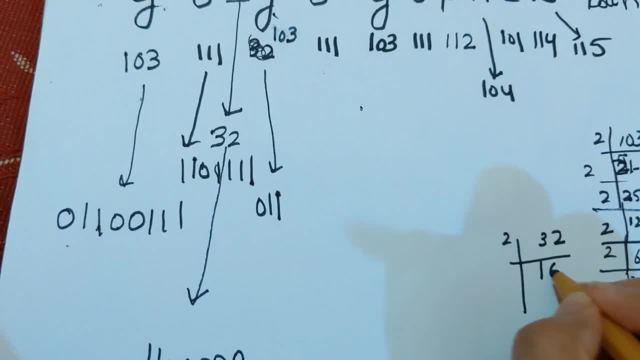 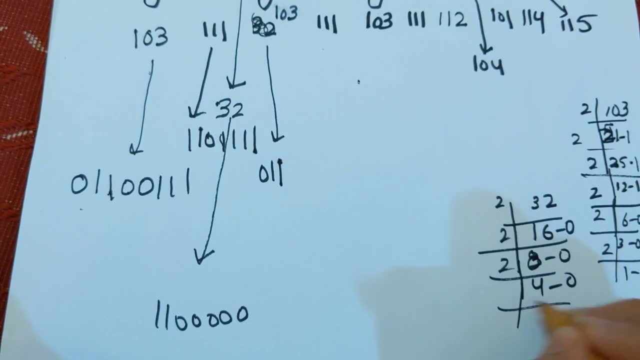 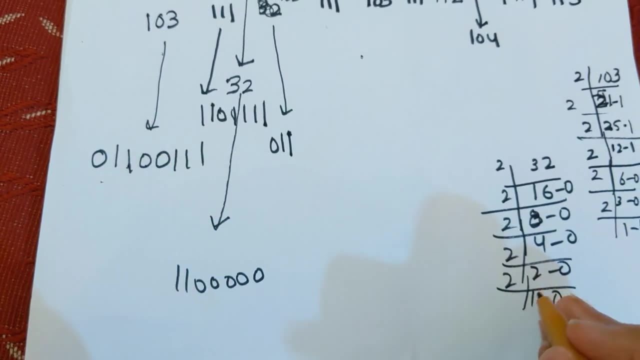 How did I know? So you should know all this: 2, 1, 0, 2, 2, 6, 0, 12, 0, 2, 3, 0, 6, sorry, 2, 8, 0, 16, 0, 2, 1, 4, 0, 2, 2, 0, 4, 0, 2, 1, 0, 2, 0, 0, 3 times 4, 5 times 0,. and what is next? 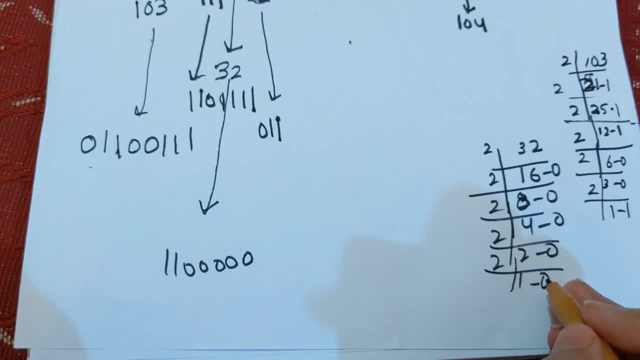 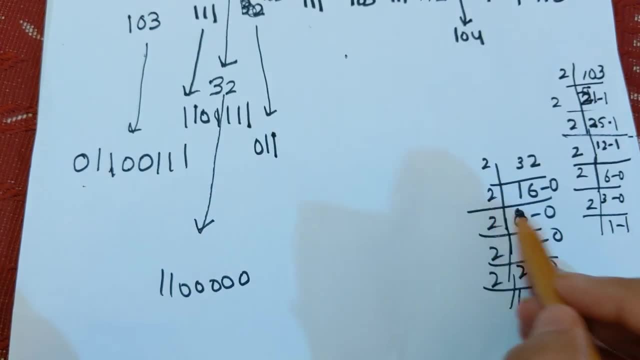 1. So here, 2, 2, 0,, 4, 2, 1, 0,, 2, 0.. Here I have taken out my perfect of 32.. It is perfect of 32.. 2, 1, 0, 2,, 2,, 6, 0, 12,, 2, 8,, 16, 2,, 4,, 0, 8.. 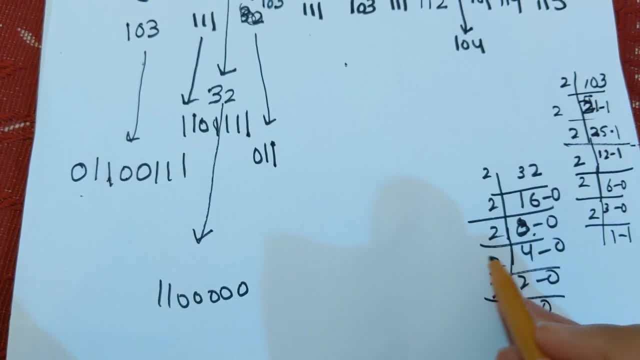 8 came after that: 2, 1, 0, 2, 2, 8, 16, 2, 4, 0, 2, 2, 0, 4, 0, 2, 1, 0, 2.. 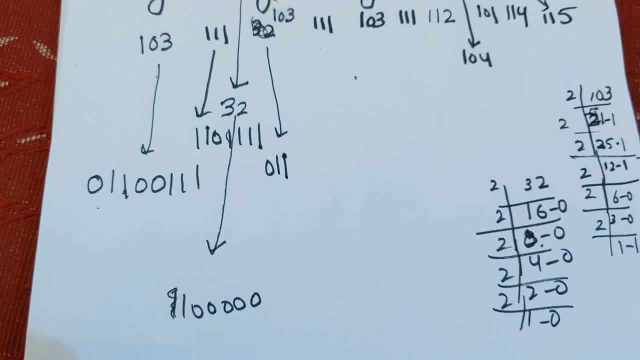 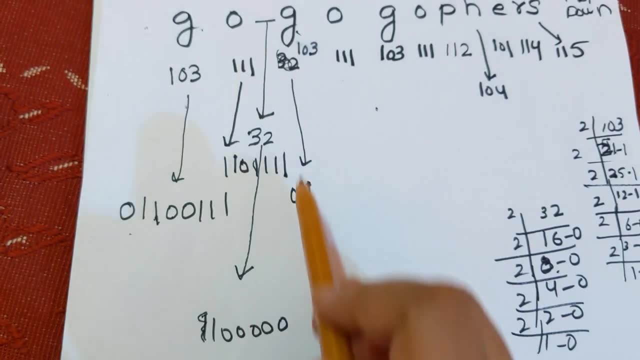 So this is our, whose. I am removing this for now. This is not it. this is it. This is your 32 binary. So we have taken out G, O, We have taken out space. Then G will be the same. 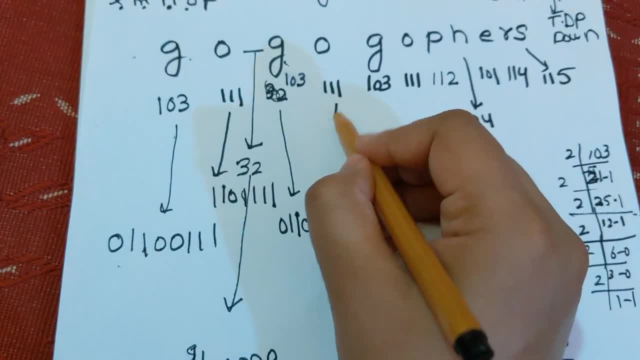 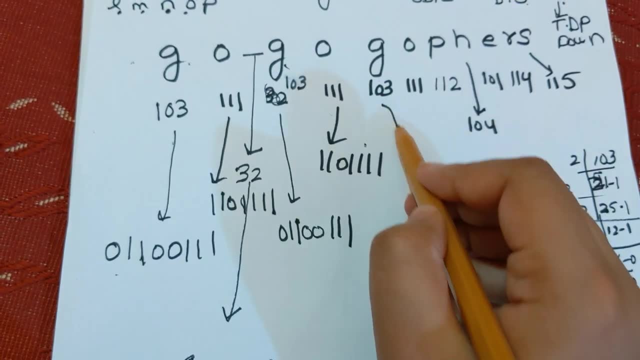 So I am copying and pasting here: O will also be the same as written here: Double 1, 0, 1, 2, 3, 4.. Okay, So in this way, what you have taken out of all this will also be the same. 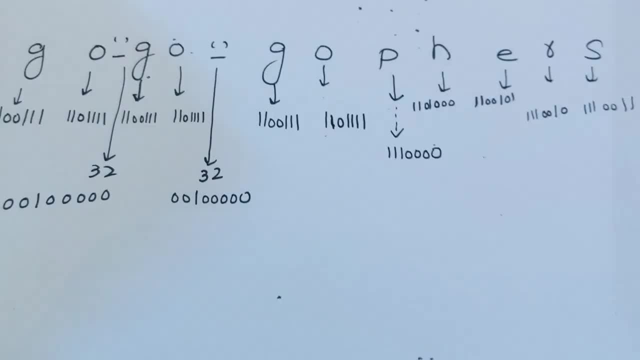 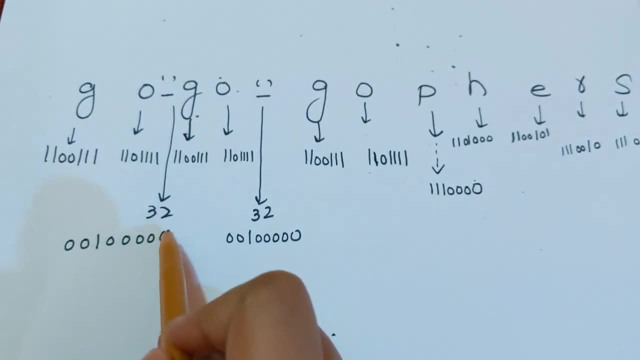 Copy it too. Now I just have to take out this. So, students, you are seeing what I have written for each character. I have taken out binary here For each character. space key For each character. space key For each character: what I have taken out binary. 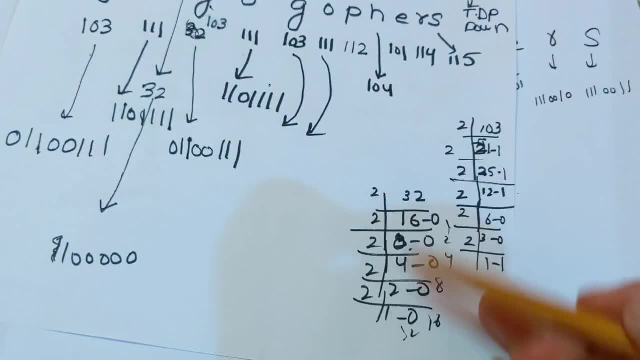 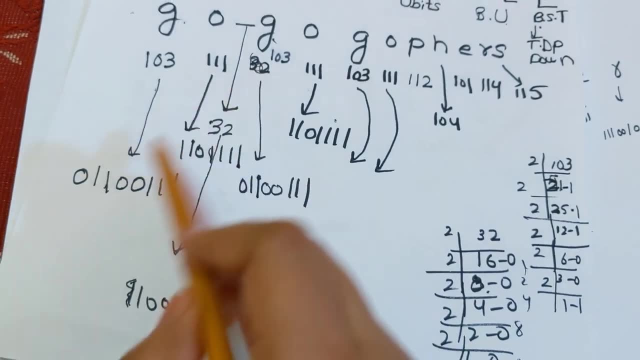 I have to take out binary. I have taught you How do you take out binary By dividing it like this. Okay, Here we have taken out G. When you divide O's Cripple 1, then it will come. Then G was same. so you copied binary. 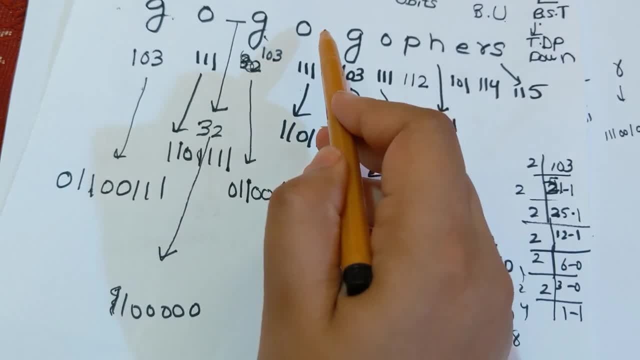 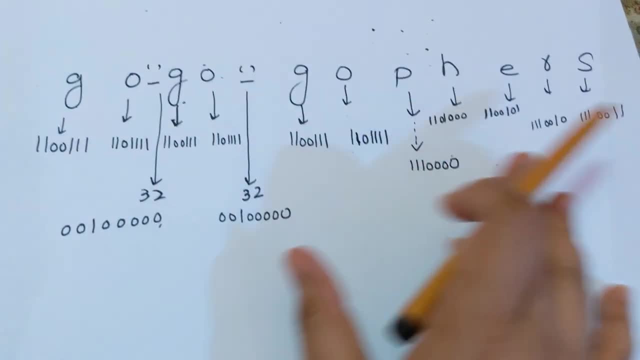 Here O was same. then you copied binary: Here space is same, Here space is also there. Okay, So what you will do, here too you will copy. So whatever binary value it had to come where I put it, I made a chart here. 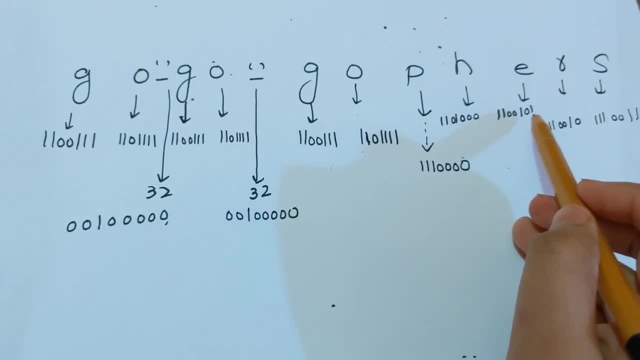 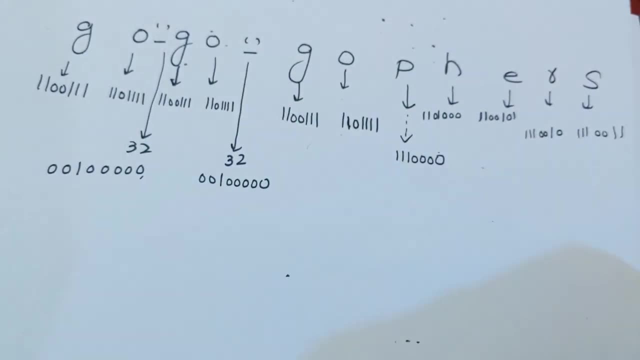 In which I have taken out everything: Binary value. Now don't get confused. Somewhere 8 bits are not getting completed, So where it is not getting completed, you can put 0 on the left side yourself. If you are not putting, then also it is automatically supposed that your bit is not on. 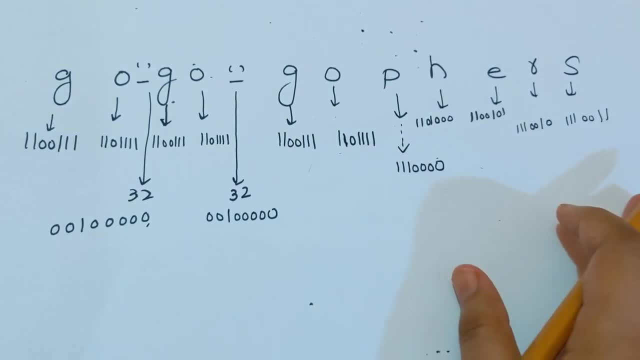 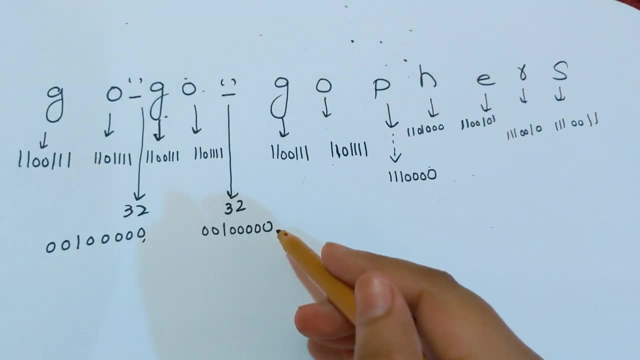 So that's why your bit is off. Okay, So what is your data? It has been encoded. So, without Huffman, you encode your data like this: How do you do it? You take out ASCII of each character, Then you convert ASCII to binary. 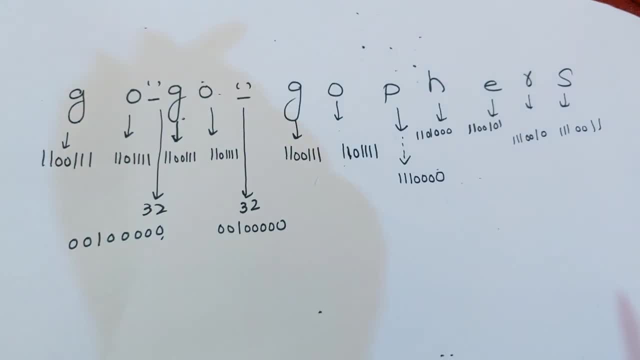 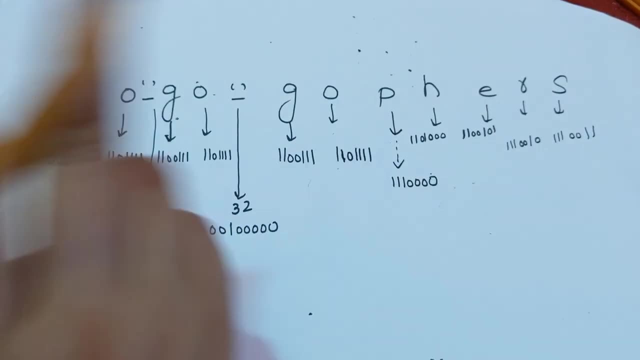 And then what happens to your data? Behind every data, your information, which is hidden in binary, it gets encoded. One thing: When you count all these bits, How many words are there? How many characters are there? Sorry, I am saying words. 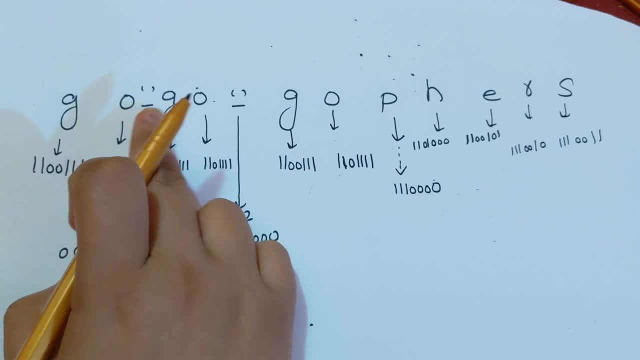 1,, 2,, 3,, 4.. Character too. Space is also a character. So 1,, 2,, 3,, 4,, 5,, 6,, 7,, 8,, 9,, 10,, 11,, 12,, 13.. 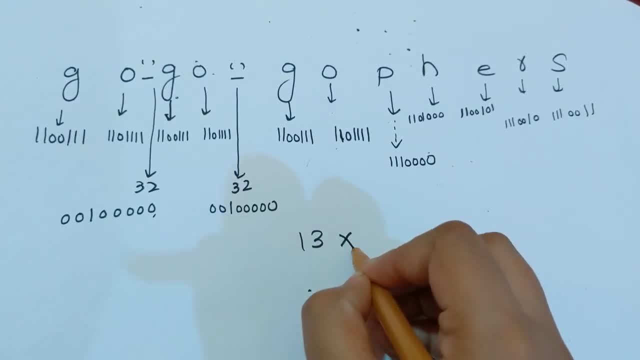 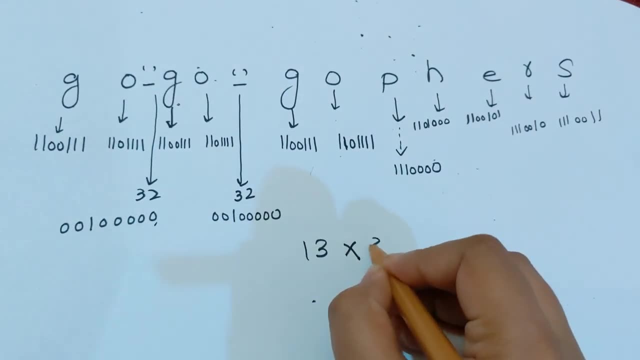 Okay, What are the total alphabets of 13?? How much ASCII does each alphabet take? How many bits does each alphabet take? 8.. So if you multiply 13 with 8, what will you get? 104.. So your total bits are 8,, 8,, 8, 8.. 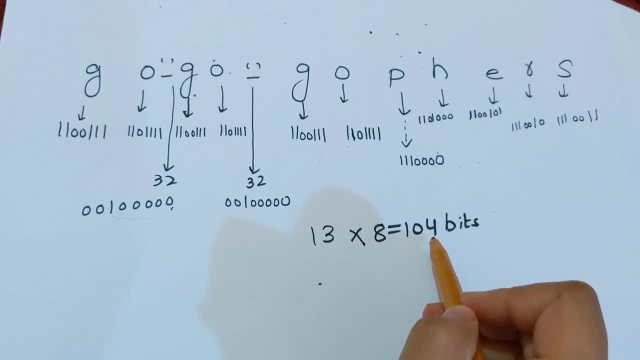 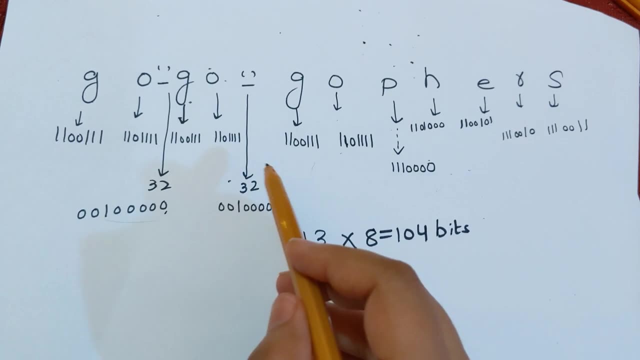 When you count all these, how many are there 104 bits. Okay, So your data is compressed. In how many bits In 104 bits? Now we will compress go go gophers again, But with the help of some new technique. 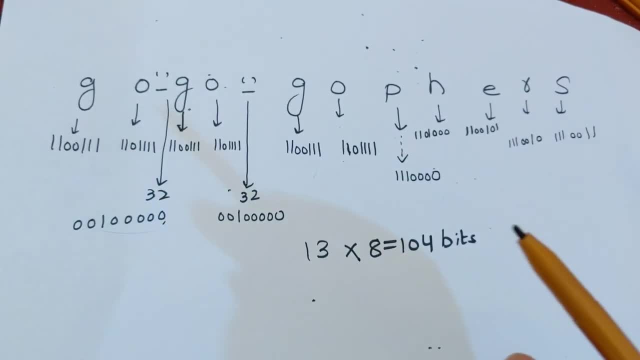 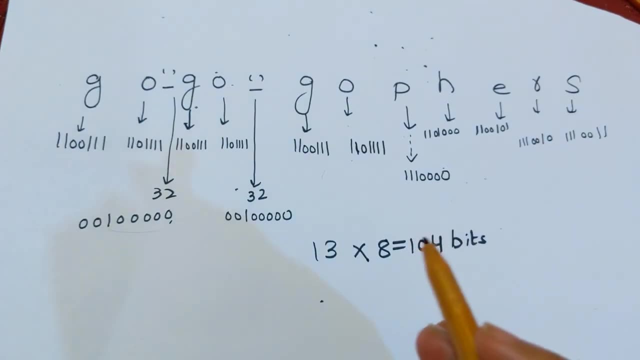 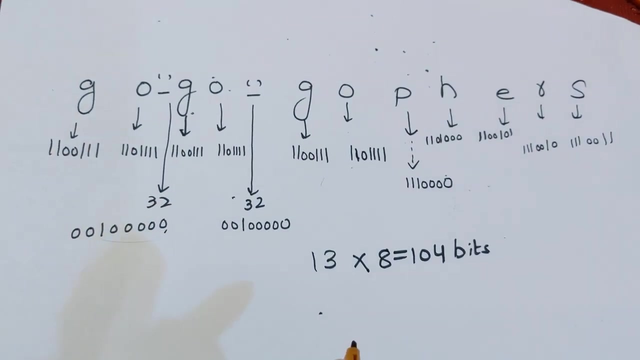 Huffman. This was our traditional work. Now we will compress this data through Huffmentry in a new way. Then we will check whether our data is compressed without losing information. Are our bits compressed? Yes, So the amazing thing is that your bits will also be compressed and your data will not be lost. 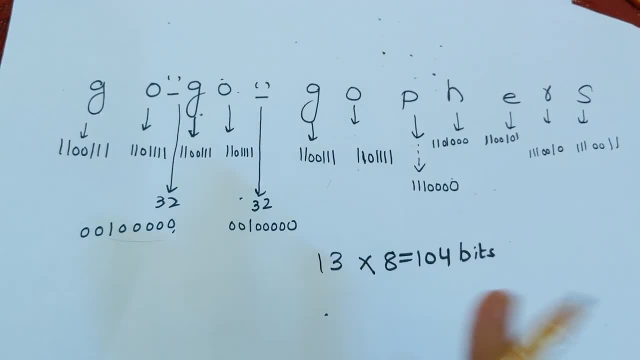 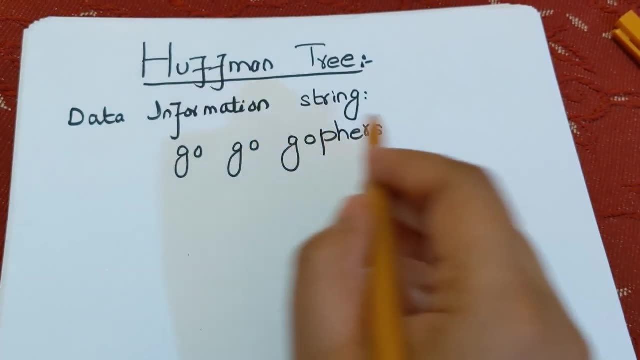 Okay. So let's see how you have to apply Huffman in this go go gophers. So what are we going to do now? Now, we are going to encode data through Huffman tree in go go gophers, Okay. 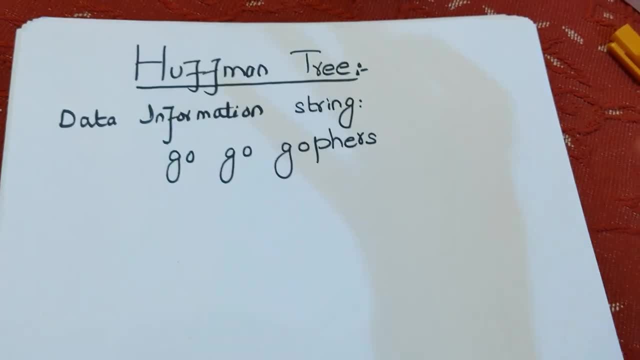 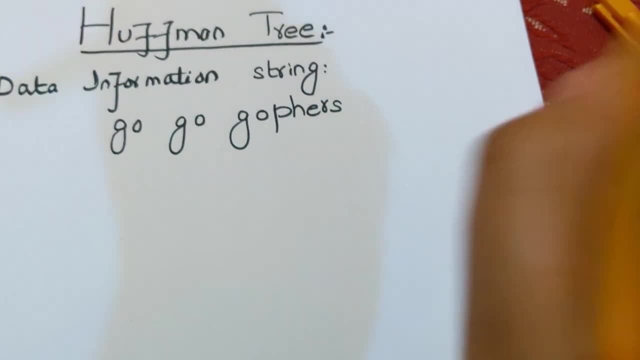 So, first of all, you have to make a frequency table, Because you know what the algorithm is. First of all, you have to count the frequency of each character, Then make a tree for each character with the stored weight. Okay, So I am repeating. 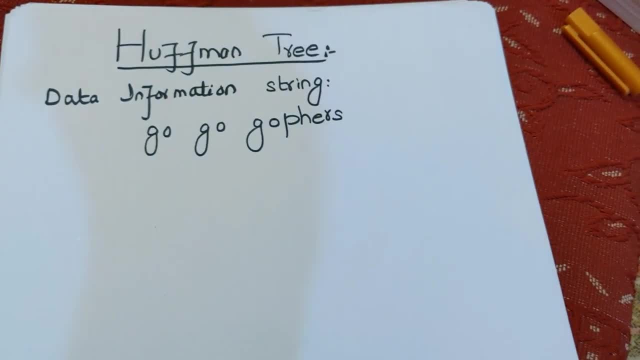 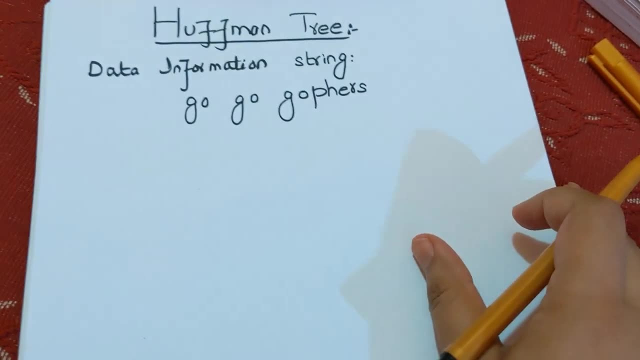 First of all you have to count the frequency of each character. So first of all we take out the frequency of each character. Then you have to take two small child, Then add them and make parent node. So let's do this. 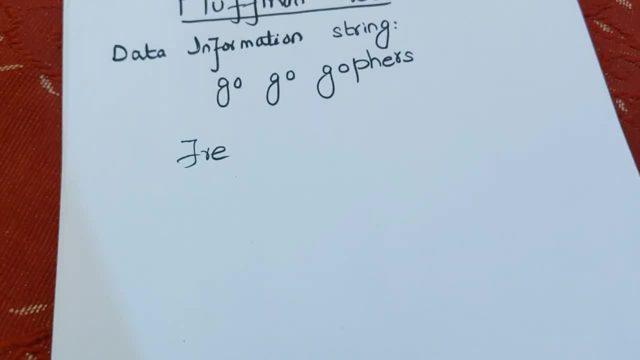 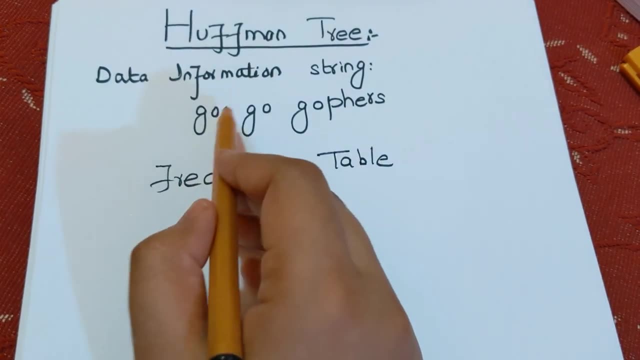 So this is your frequency table. I am designing it here. I hope you guys are getting it. Our frequency table has been a little love up procedure, So in the frequency table you have to write the occurrence of each character. How many times has it occurred? 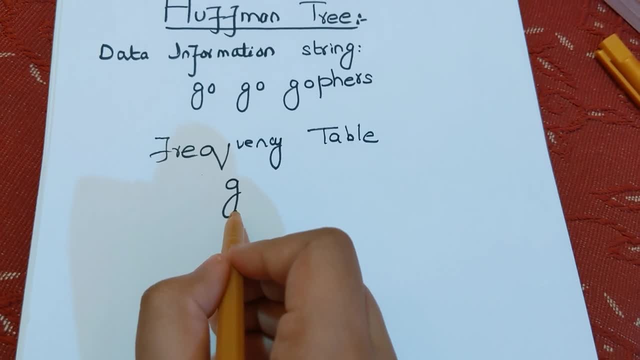 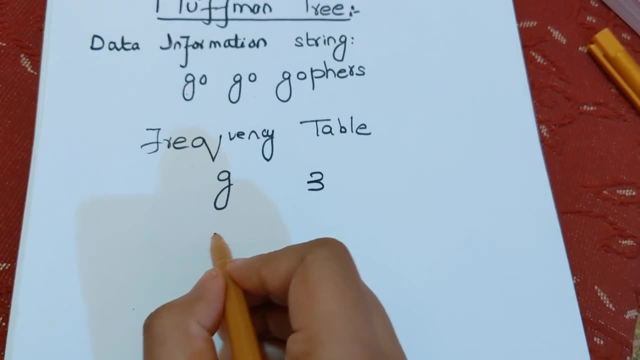 So G, No matter how many times it has occurred, I have written G only once. I have added G in the frequency table. G is my character. What is its frequency? Three times One, two and three. After that there is your Go. 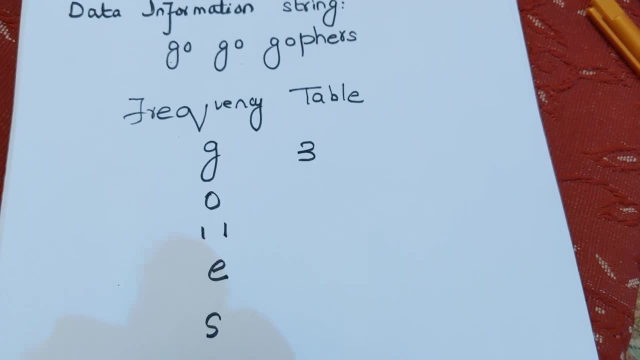 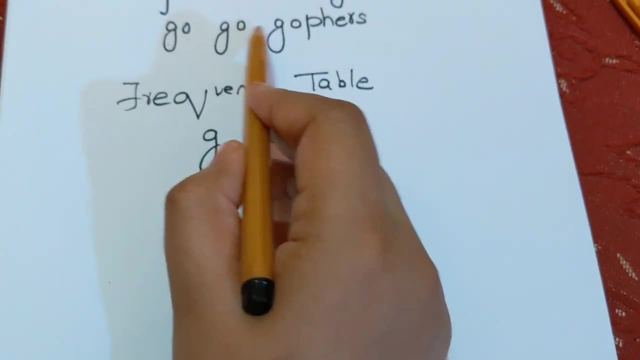 There is your space character, There is your E, There is small s, There is H, There is P And then R. So now I have to check how many times my O has occurred. So you can see O is one, two, three. 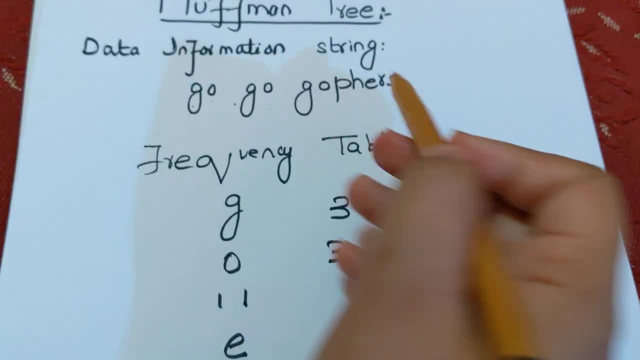 It has occurred three times. How many times has your space occurred? Your space is one and then two. Your space has occurred two times, So here is two Now. what is yours Now? it is E. How many times has E occurred? 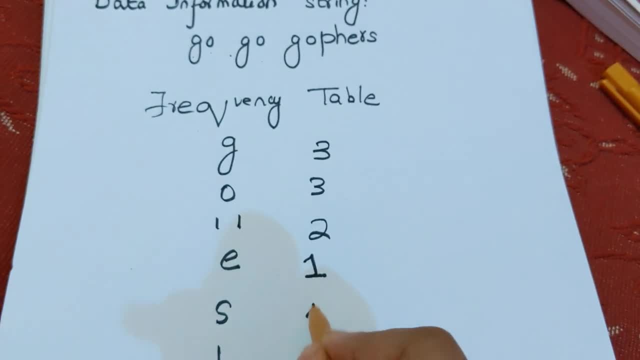 One time, Sb One time, Hb One time, And here is your Pb One time. So what frequency table has it become Now? what do you have to do through this frequency table? You have to make a Huffman tree. 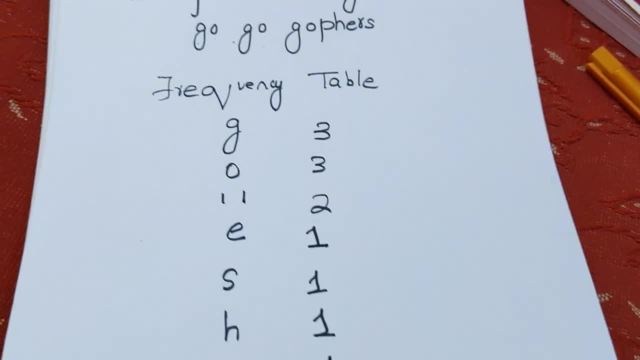 Okay, so now we are going to make a Huffman tree. You know that you have to prioritize whose short length is, I am sorry, Short length. Now you say What is its low frequency? You have to make a child node for the low frequency. 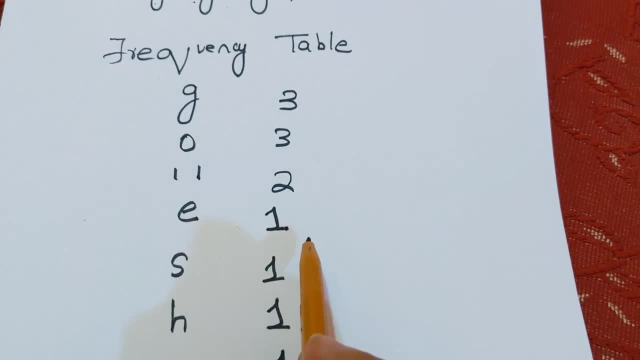 So what do you have to do? by making these two? You have to design a parent node. This is its frequency, This is his, This is its, This is its, This is its And it is a child node. So we have to choose. 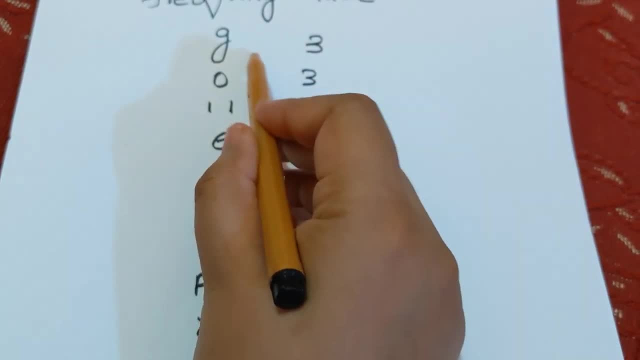 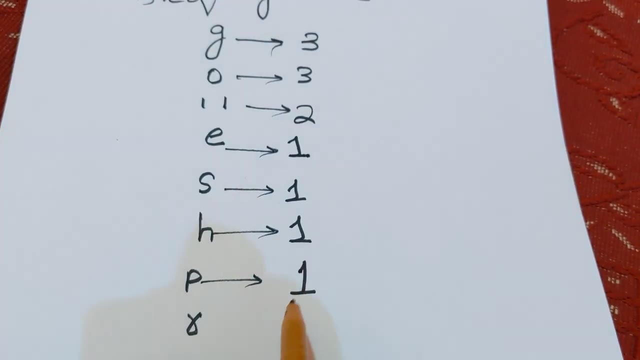 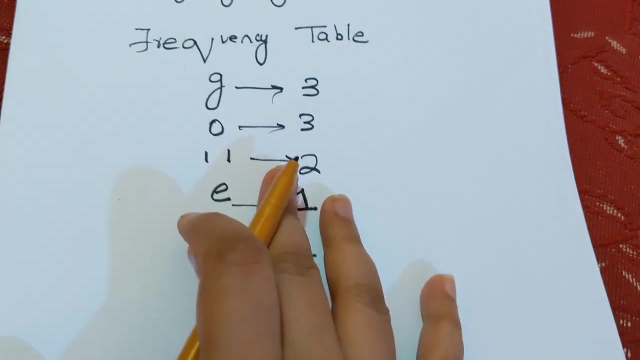 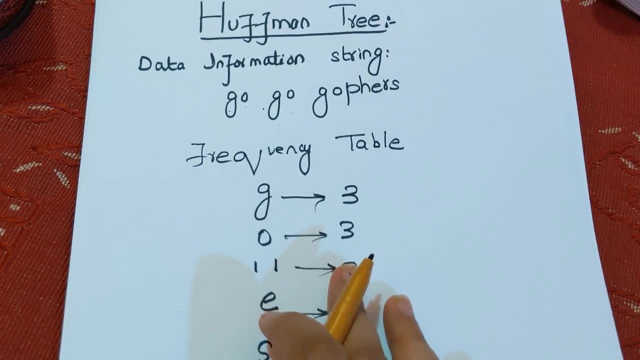 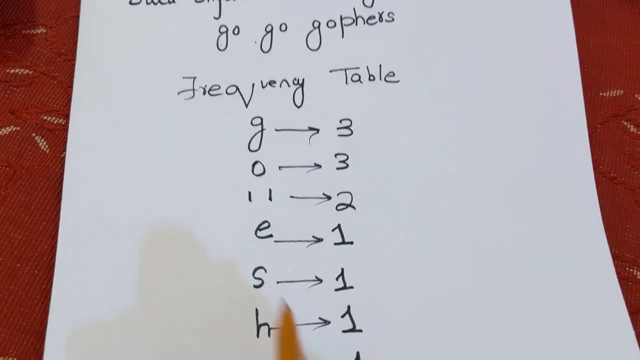 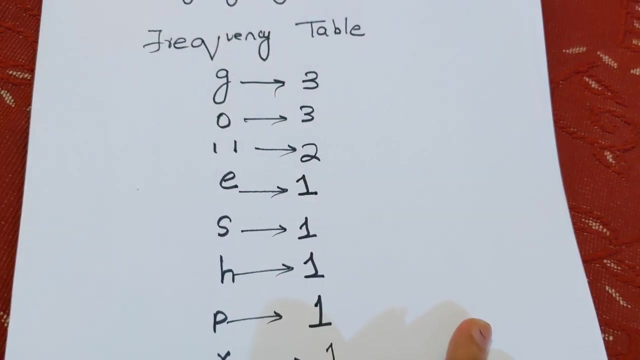 tree, binary search tree is kept. okay, binary search tree or binary tree. and in Huffman tree we put priority queue. Why? Why did I say priority? Because you see the priority whose frequency is low, you start bounding it from there and merge it. So here the low. 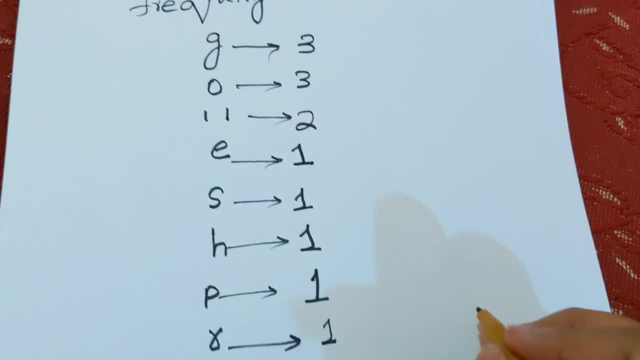 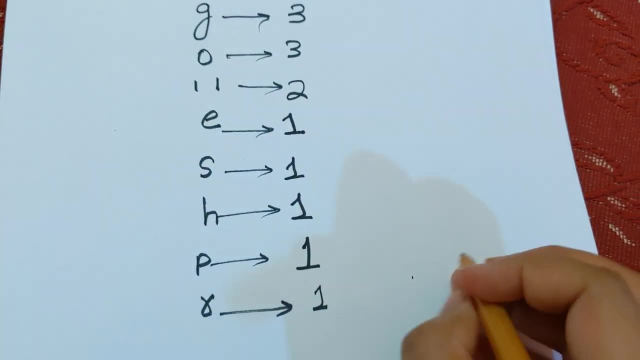 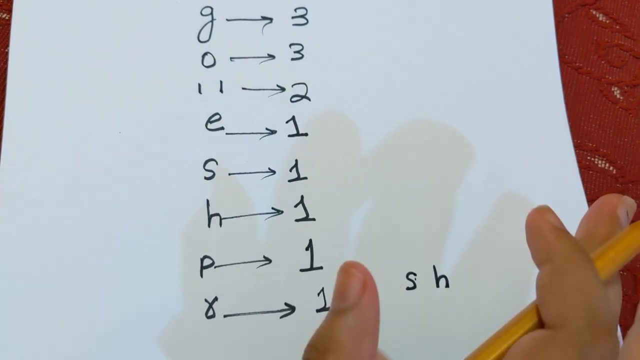 frequency is of everyone. so see what I do. let's take everyone in two nodes. so first I take SE or SH, whoever you want to take, then take PR, it is up to you. so I do this. I take SH, I took SH, let's spread both. okay, whoever you want to take, it is up to you. 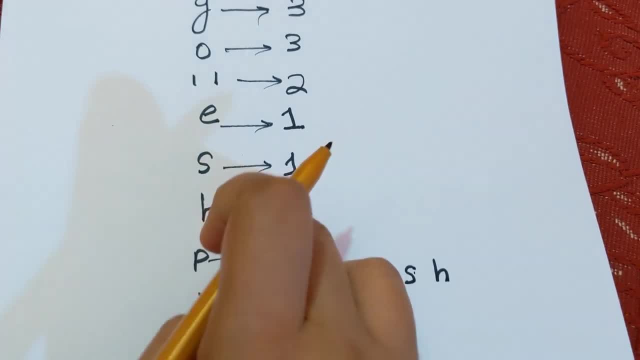 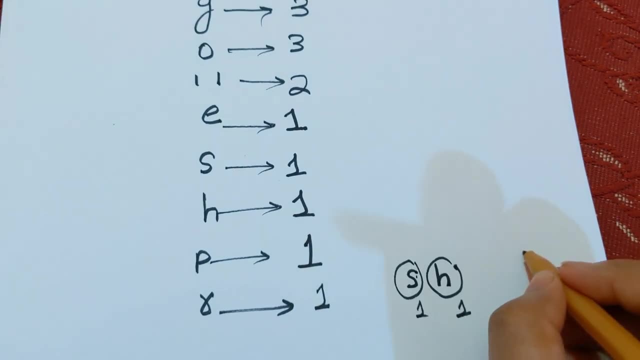 you take both of them. you take both of them. leave it. you take both of them. you take however you want to take. it is up to you. so I took S and H. you don't have to get confused at all. both of them had one frequency. then I took P and R. you could have taken ES as. 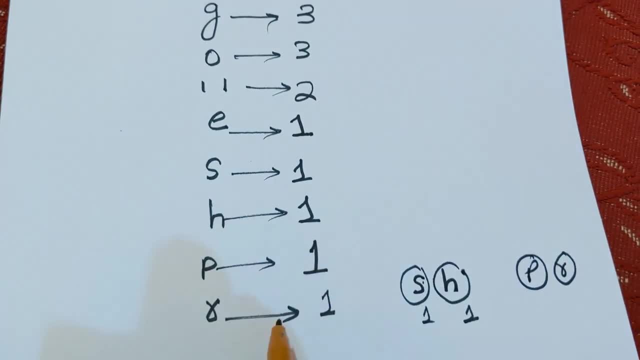 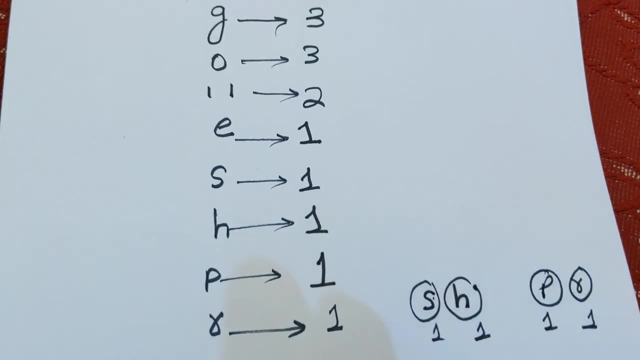 well, E also had one frequency, so you randomly take whoever you want to take, because everyone has a low frequency, all the lowest ones are in it. so this is it. this has become two parent nodes because our algorithm also says that after calculation of frequency, it is 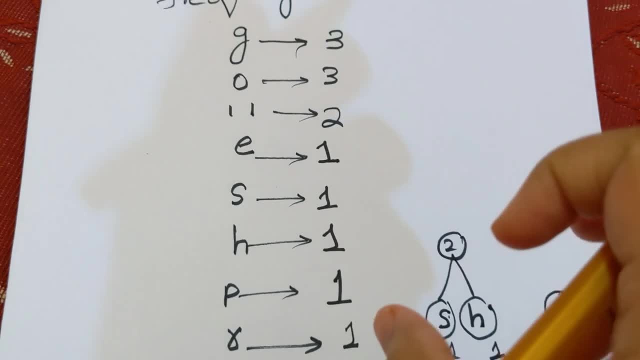 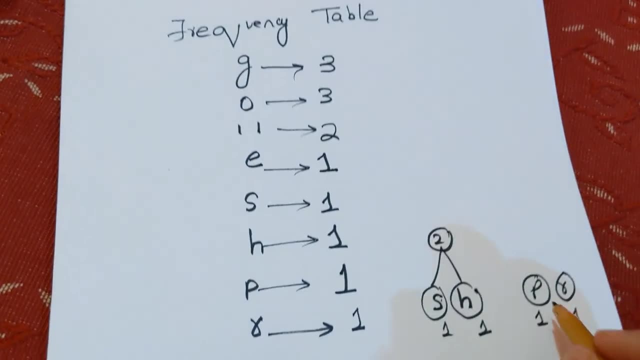 a frequency. what you have to do? you have to pick two child nodes and sum them up, and you have to keep doing it until your list is empty. your entire data is not traversed. so if you take this one one, then what is our two again, what is our two, two after? 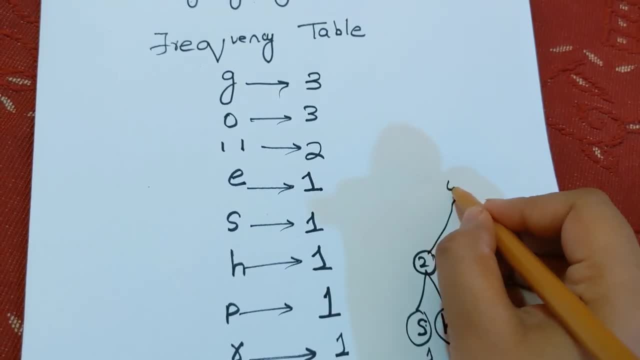 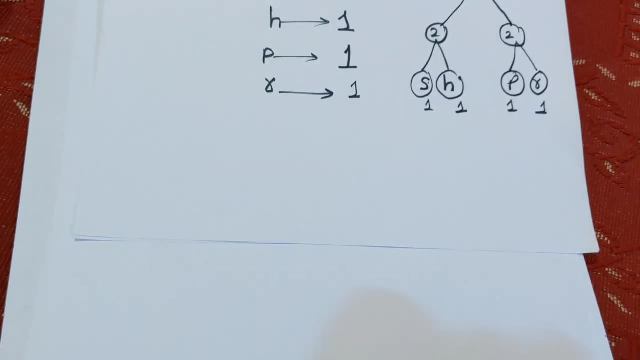 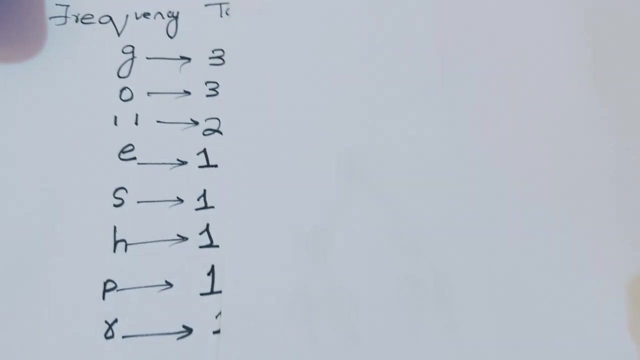 building four. okay, so I would like to do this thing again here so that you guys can get more clear. I have kept this page in front of me of frequency, so first of all I checked who has the lowest frequency, so I got the lowest frequency. who got it? all of them got. 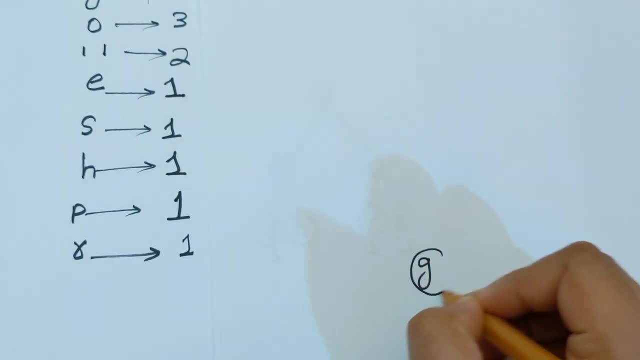 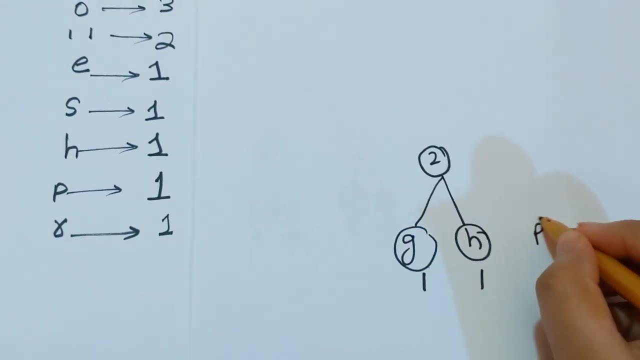 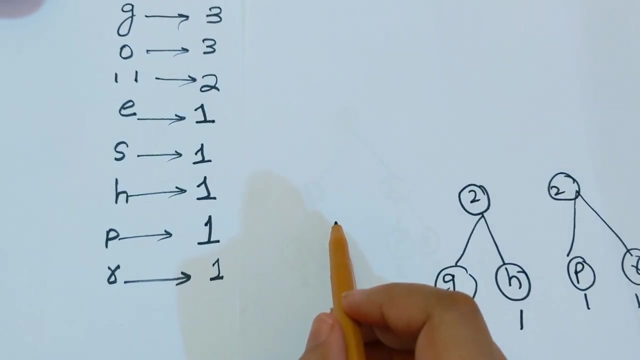 it. so what did I do here? I took G, took H, and because both of them had one one frequency, I summed them up then it became two. then I took P and I took R. both of them had one one frequency. I summed them up, then it became two. okay, now I checked that after doing 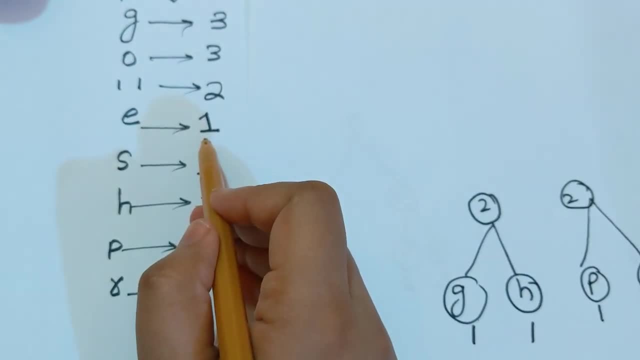 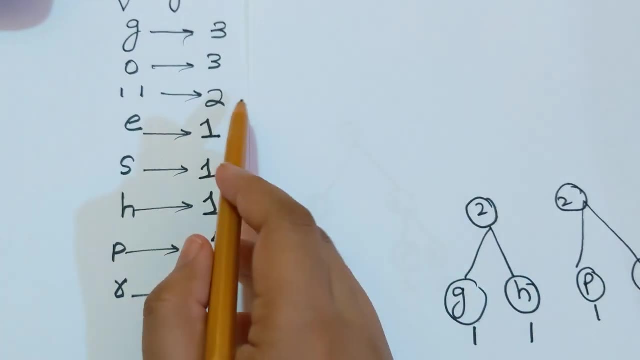 this work. now my E is saved. what is the frequency of E? it is one. okay, one frequency. apart from this, there are two, two, but whose frequency is lower two. so I have to pick two again, child node. so let's do one like this, let's merge it with two, let's take 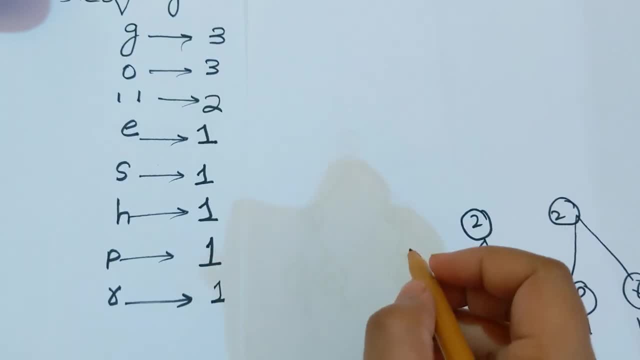 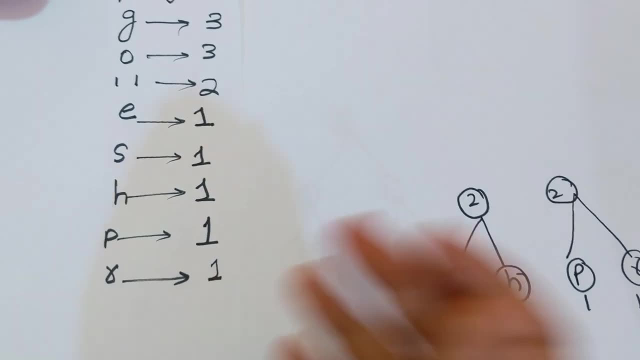 these two too of the character. so I said that I am taking one and two, so you can take as you want: take two one or take one two. if you want, then you can put a binary search tree algorithm in it that you said that I will keep small on the left and big on the. 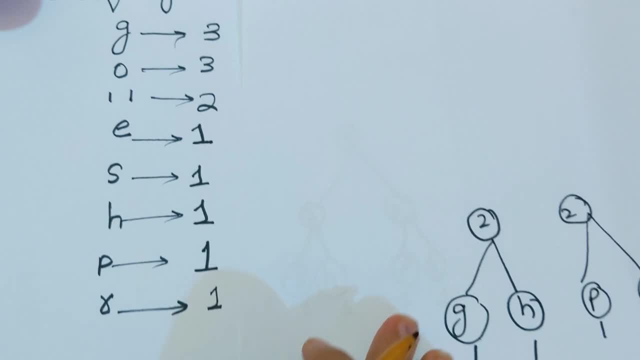 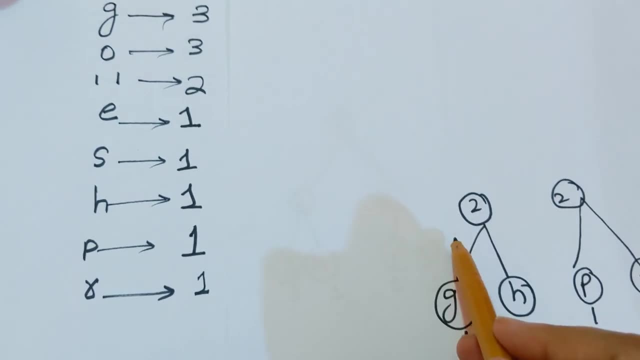 right, or you just keep it as a binary tree. there is no harm, okay. so I am trying to convert it. that in which In binary search tree algorithm. so, because I know what happens in binary search tree: small on the left and big on the right. so see what I am doing now. what I did, I made. 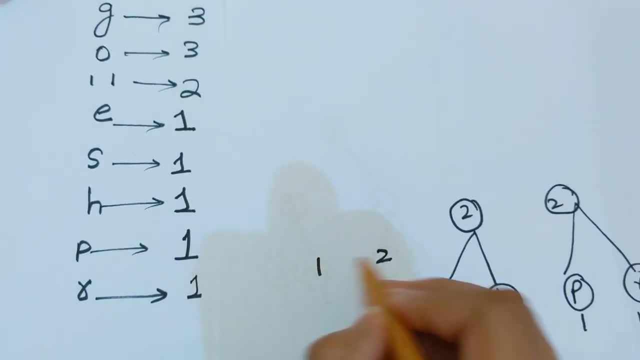 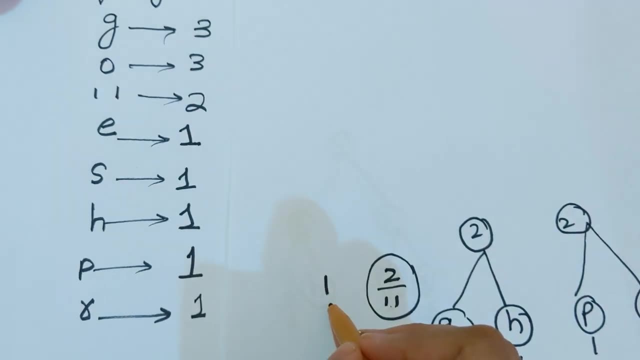 three. I took two on the left and took one on the right. that is, I took space on two. okay, this is your space. do it like this. this is your space. and whose was this one? your E? so, these two together, because both of you were small nodes, these were small. 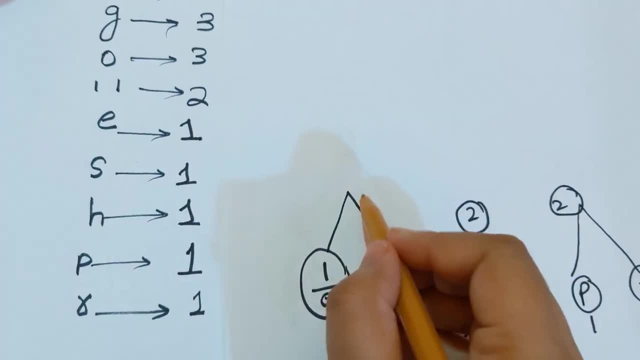 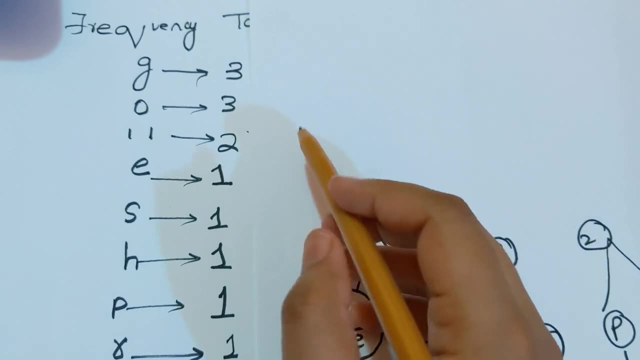 frequency characters, both of you. you took both of them. what became your three? now? you have checked that. there is three. there is two, two, whereas what is in your frequency table? there is three, three. so for now, two, two is very small. three, three, we cannot. 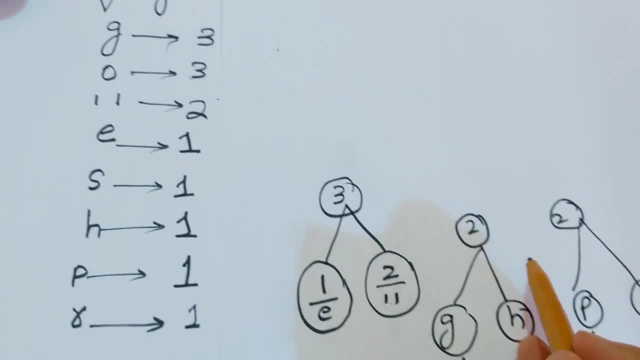 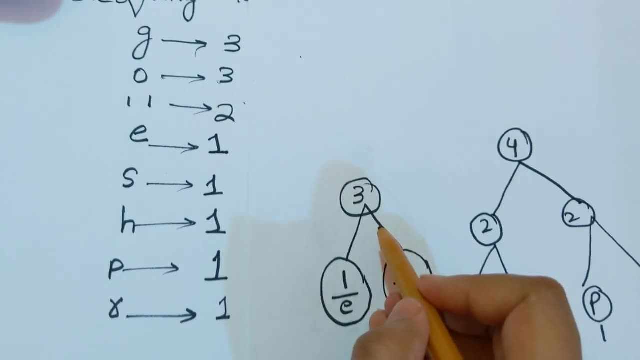 take this too. we cannot take this too, we cannot take this three too. so first, what we are getting small, what we are getting, we are getting two, two. first we merge these two, so this became four. now check, so this three, this three, this three is smaller than. 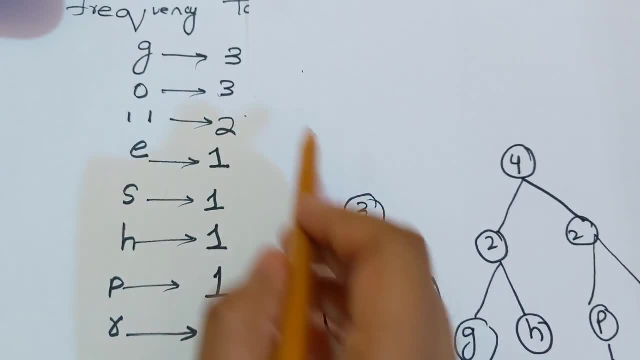 this four, so we do not have to sum up this four now. I put it aside. first I take these two three. okay, because what are these two three? My two child nodes can be made very easily. so I took these two three. so see here it. 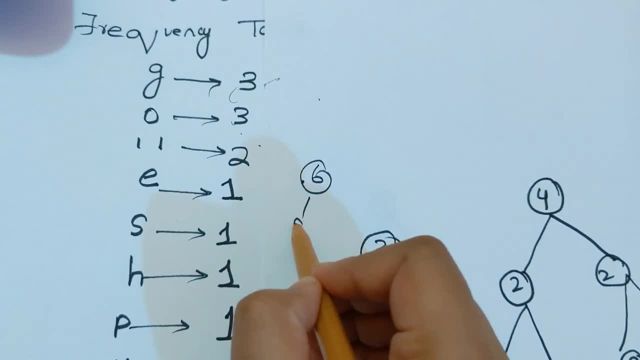 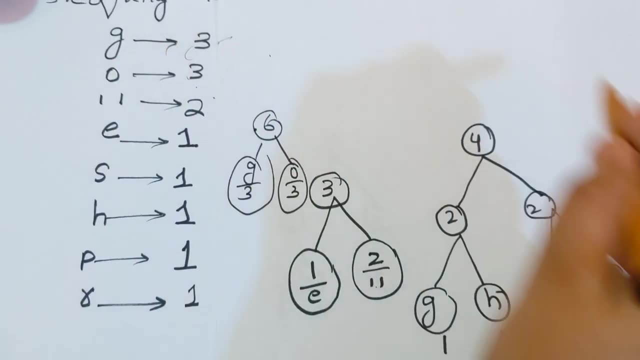 came, it became six. I took three in this G, and what did I take in O, three, so this became six. so I have completed this. now I am combining the tree, I am summing up. so this is small, this is big, this is small. that is, these two are your small nodes. 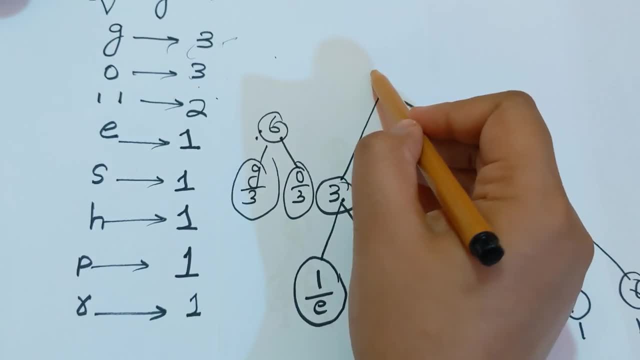 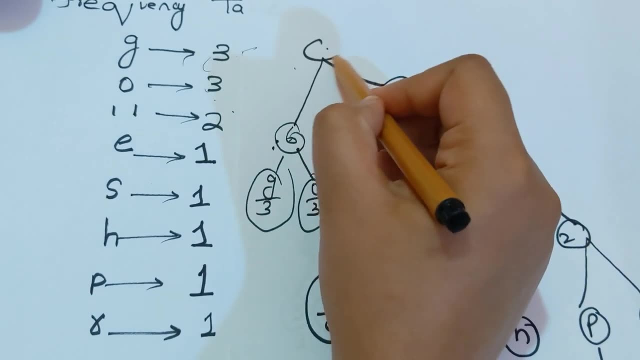 so you sum up these two. what is four and three? Your seven. see again, now you are here. six and seven are your last child nodes. so you sum up these two. what is six and seven? Thirteen you count were your characters thirteen. 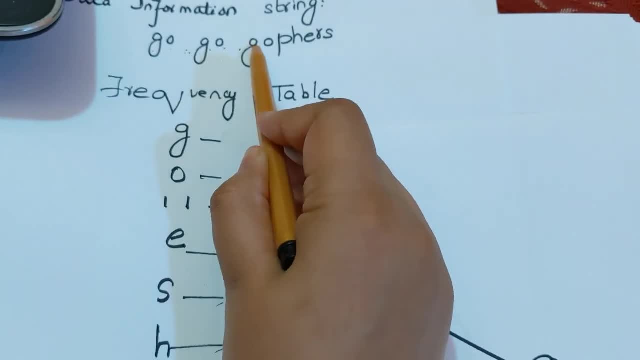 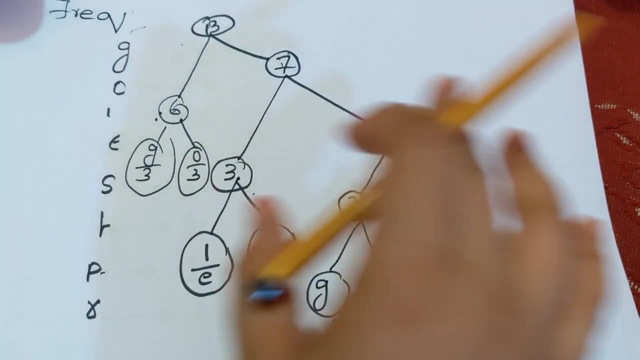 One, two, three, space, four, five, six, seven, eight, nine, ten, eleven, twelve, thirteen, yes, thirteen. so sum up, your answer is thirteen. if you did not understand my tree traversing. 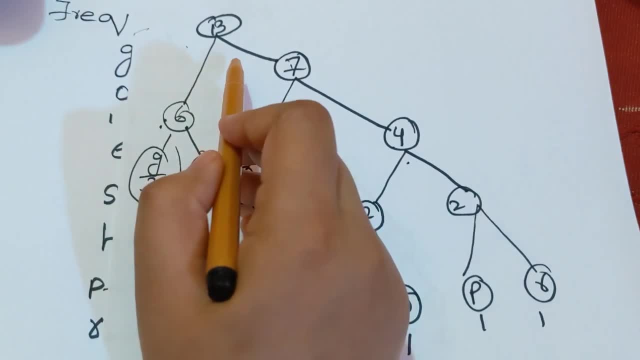 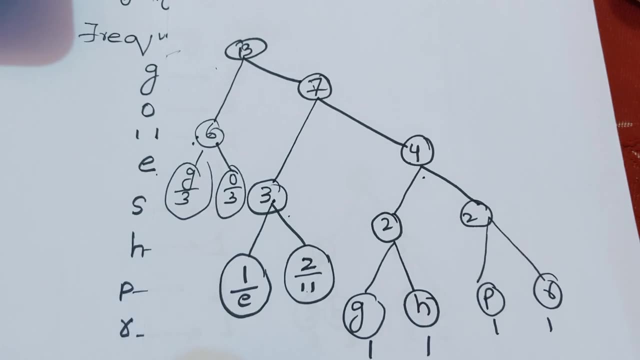 then you made a tree in your own way. you check, then only your answer will be thirteen. okay, now, what will we do in this Coding scheme? now we will encode in this. do you know how we encode? So how do we encode? 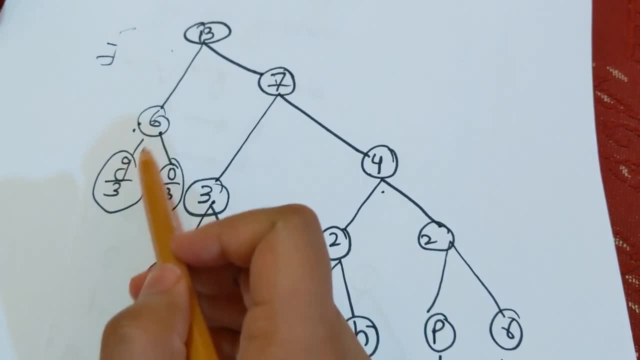 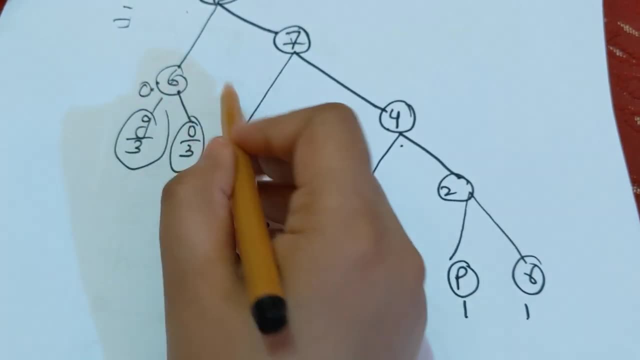 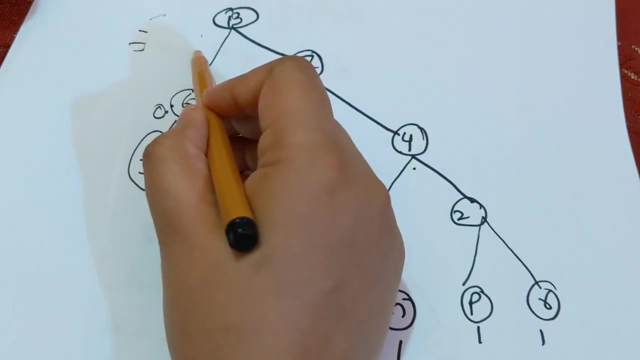 Read: every left turn is zero and every right turn is one. so what did I say? Read: every left turn is zero and every right turn is one. so you put one on zero, left on zero and one on right, left, zero, right one. 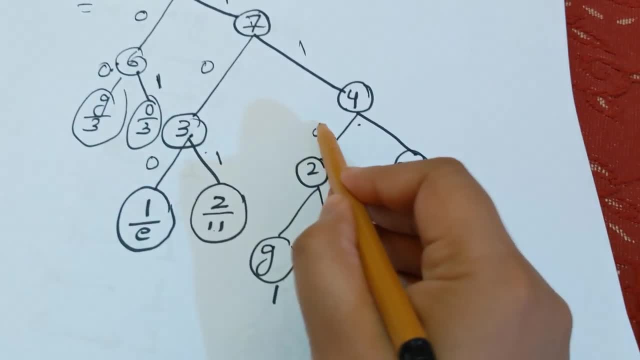 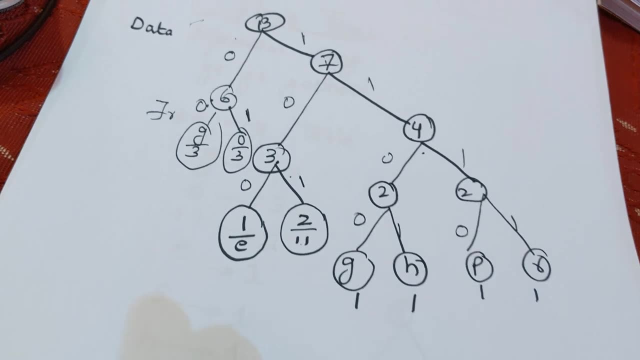 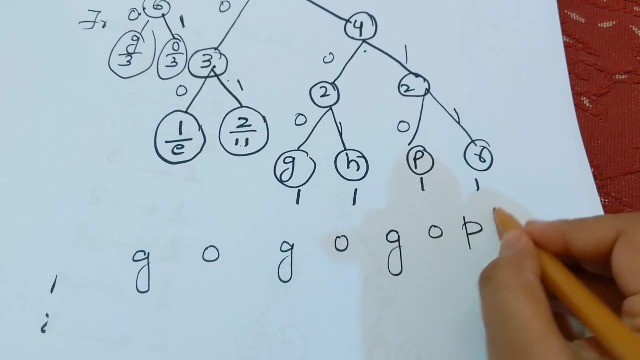 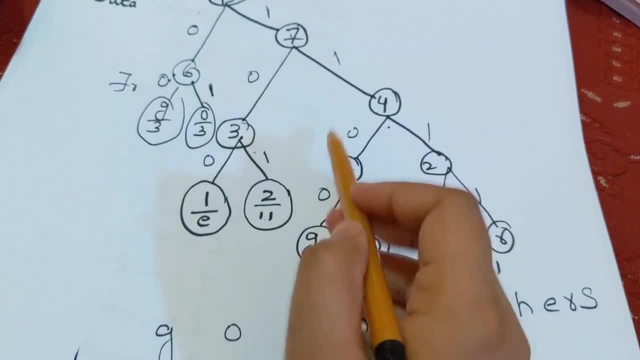 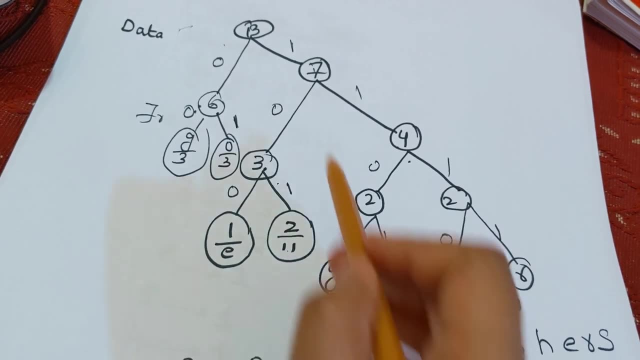 where does the traversing start From your root note? okay, how do you have to traverse? Root to note, root to note, which note do you want? so you have to write that part in which your traversing starts from the root to the note. 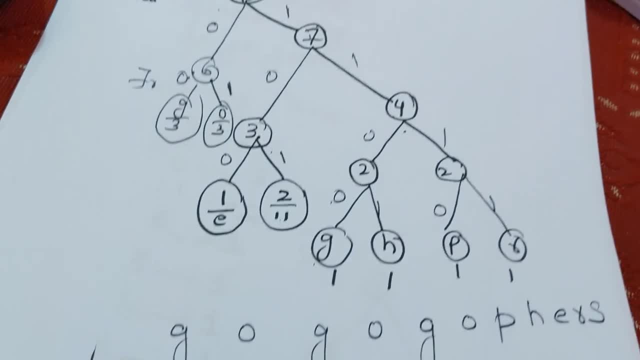 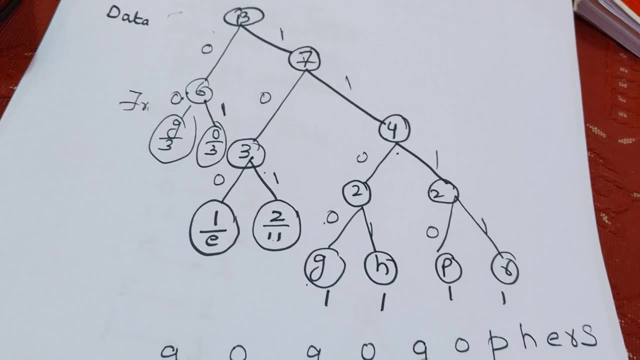 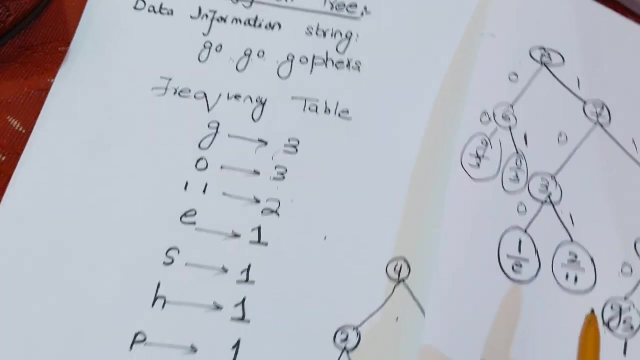 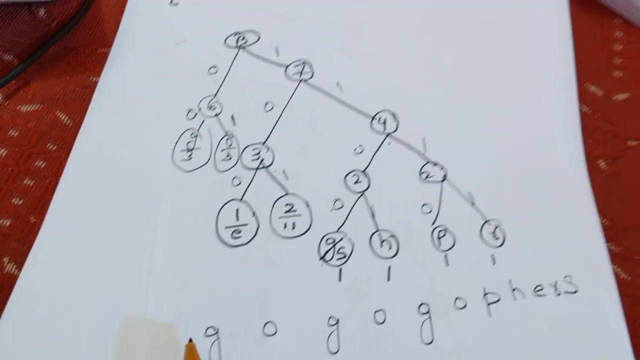 so one, one, zero, zero. then what came? I think I am wrong. I am telling you wrong. I am repeating again here. I think I had to write S here. here I wrote G, here it was S, because you see, here it was S. now it is correct, this is your S, this is not G. so again I am repeating: where is G coming? it is coming here. so what is 0, 0 in G? so you have written here: coding scheme 0, 0,. 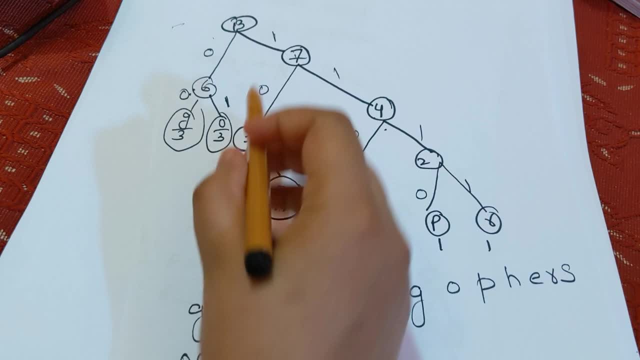 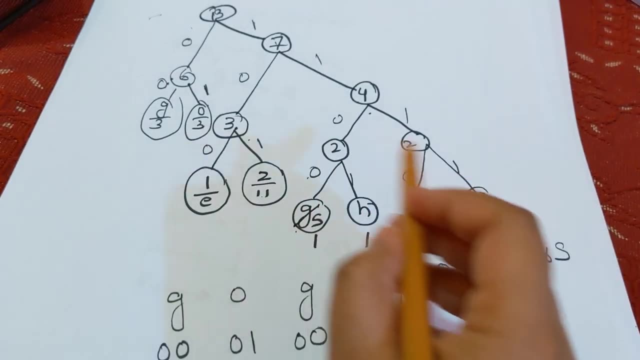 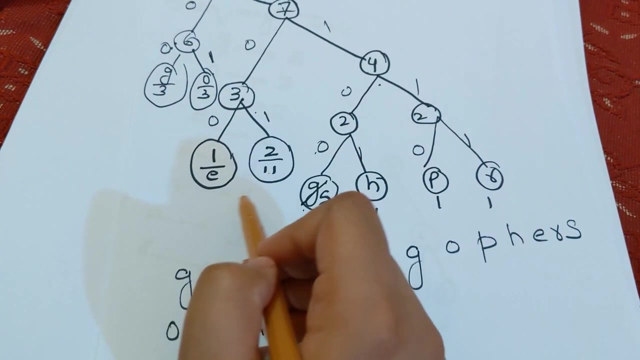 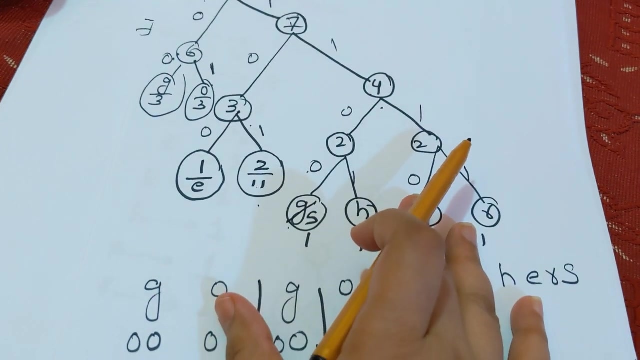 O. where is O? what is O? root to leaf: 0, 1,. so you have written 0, 1,. if it is repeating again, then check 0, 0,. where is G coming? it is 0, 0,. let's see space. where is space? it is here. where did you start? from root to leaf node 1 0, 1,. so what is your space? 1 0, 0,. let's see again. 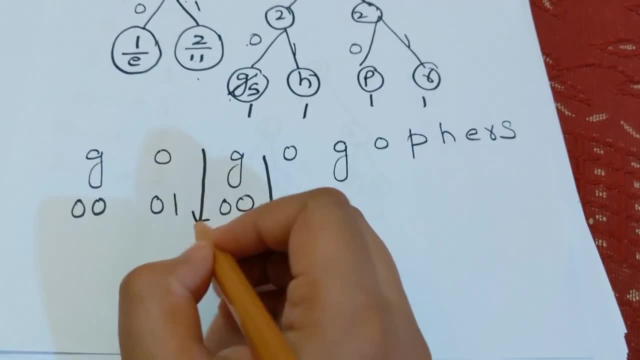 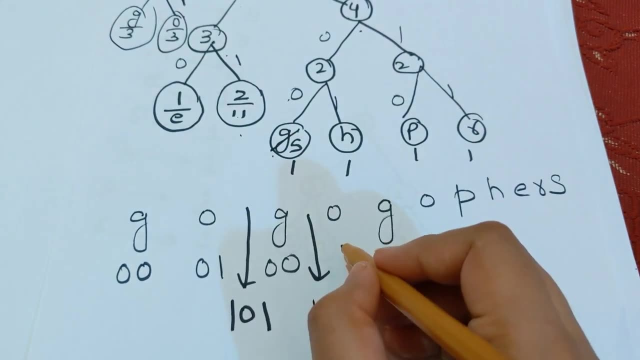 so what is your space? 1 0, 1,. so here it is 1 0, 1 space. then space will come here: 1 0, 1, here it is 1 0, 1,. your O is repeating again, that's mean 0, 1, I have copied. G is repeating again: 0, 0,. 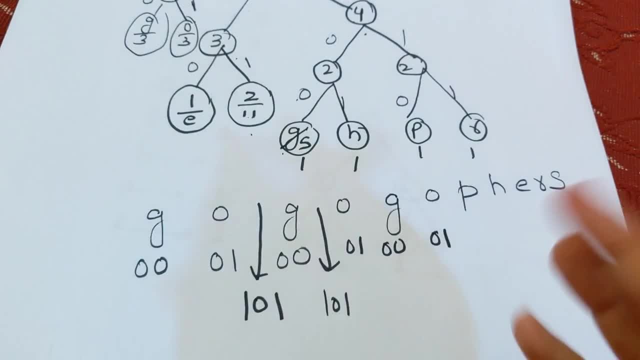 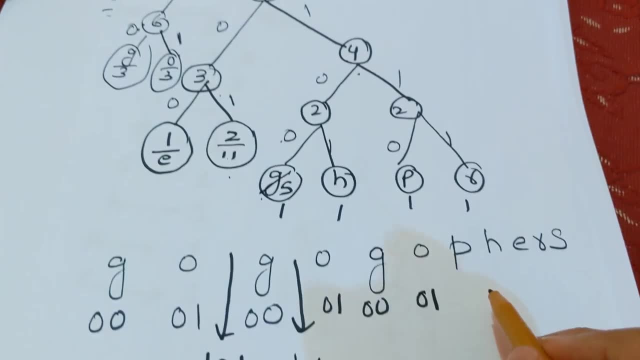 now what is O? repeating again? that's cool. I took this example knowingly so that data doesn't have to work hard and get solved quickly. P- see P is coming here- 1 1 1 0,. so what is P? 1 1 1 0,. what is H? see 1 1 0,. 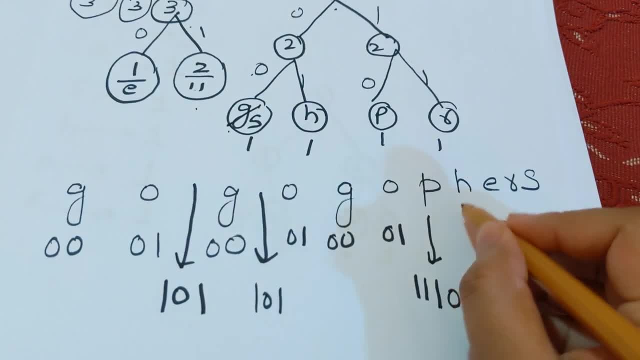 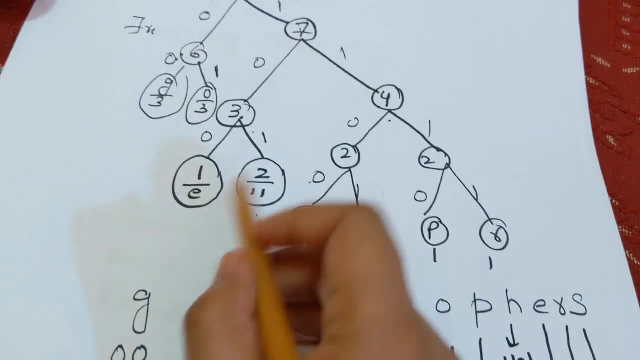 1 0, 1,. so what is H? I am writing here 1 1 0, 1,. what is E? what is R? what is S? so first I will write E. where is E? it is here 1 0, 0,. 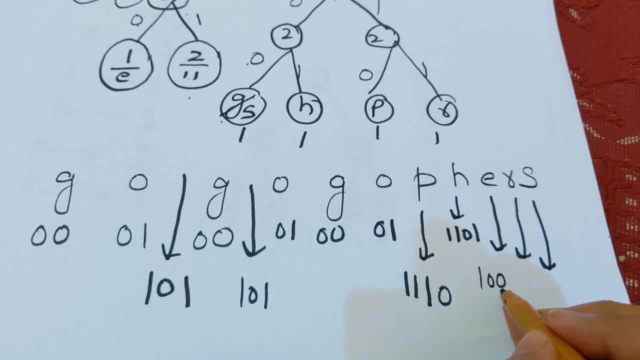 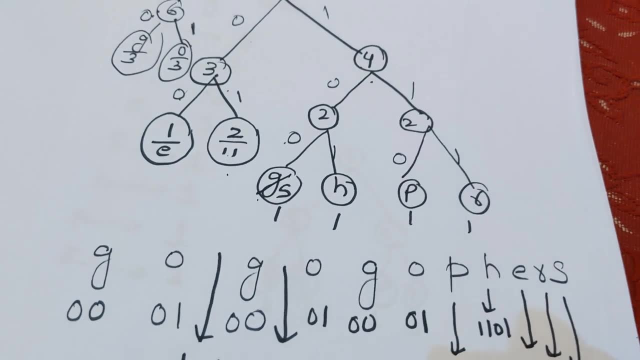 E is here. 1, 0, 0,. ok, and we have now what is R? R is here, R is all. my 1, R has 1,, 2,, 3,, 4,. see how much is S. where is S? it is here. 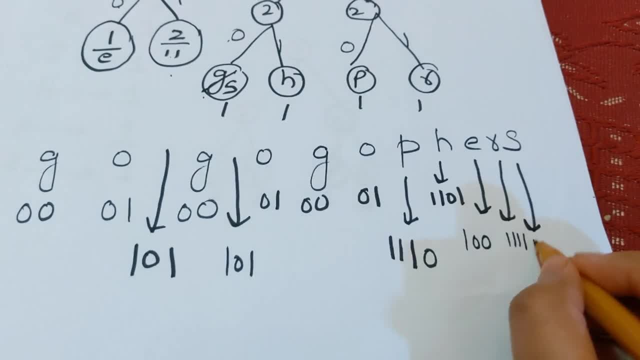 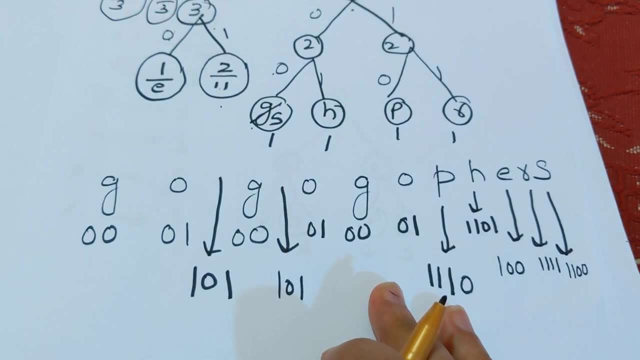 1 1 0 0, 1 1 0 0,. note one thing: this is your encoding scheme. ok, note one thing: that when we, when we did previous work in that every character was taking 8 bits, 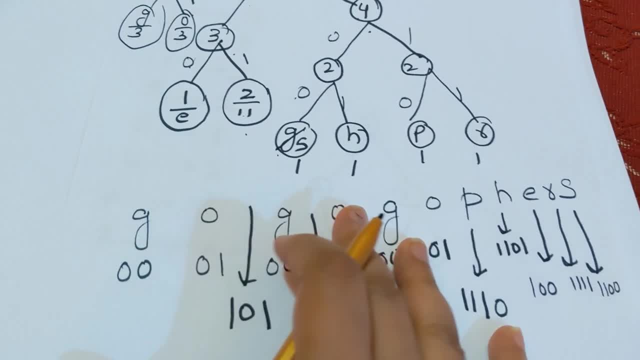 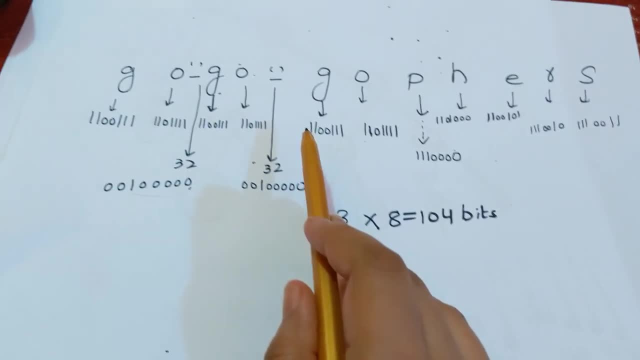 total, we had 7 characters. ok, so 13 characters, not 7, 13 characters. we had, as I told you here, 13 characters, and every bit, every data, takes 8 bits, every character takes 8 bits. 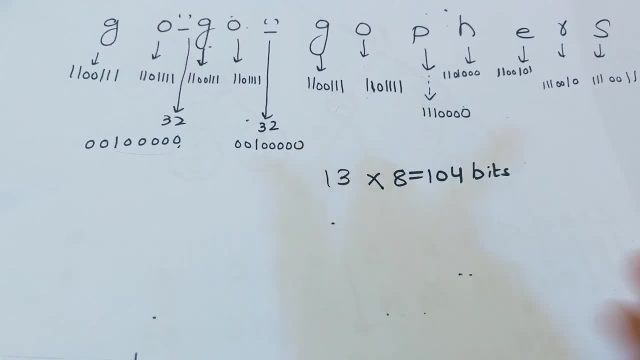 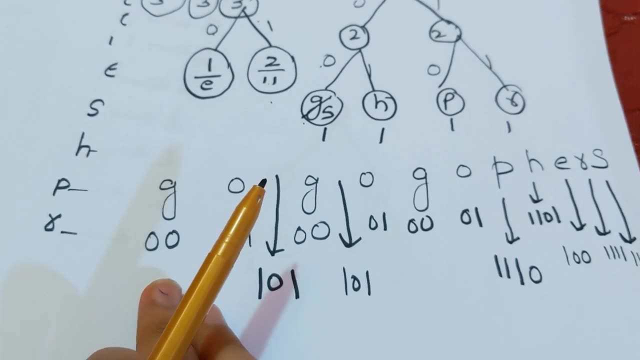 so 13 multiply by 8, how many bits did you make? 1 0 0,. 1 0 0 0, 14, 14, in total, 4 bits here see, every character did notиров 8, 8 bits' data. your data is compressed here: whosoever took 2 bits, someone took 4,, someone took 2, in short, your data is low. 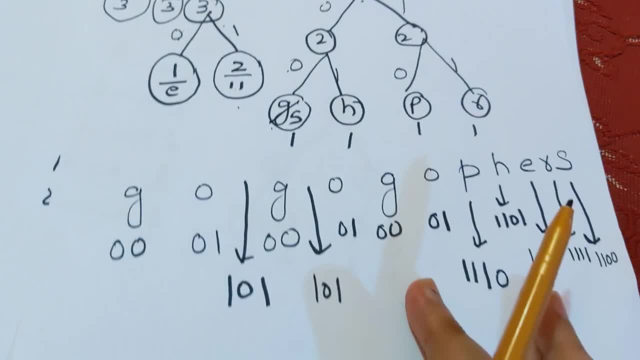 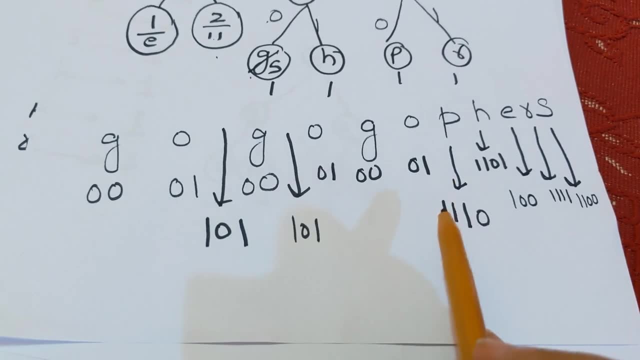 8 bits. it did not work and even your data loss has not taken place. now you count this: 1, 2, 3, 4, 5, 6, 7, 8, 9, 10, 11, 12. I am counting again: 1, 2, 3, 4, 5, 6, 7, 8, 9, 10, 11, 12,, 13, 14, 15, 16, 17, 18,. 1, 2, 4, 4, 5, 6, 7, 8, 9, 10, 11, 12,, 13, 14, 15, 16, 17, 18,. 1, 2, 3, 4, 5, 6, 7, 8, 9, 10, 11, 12,. 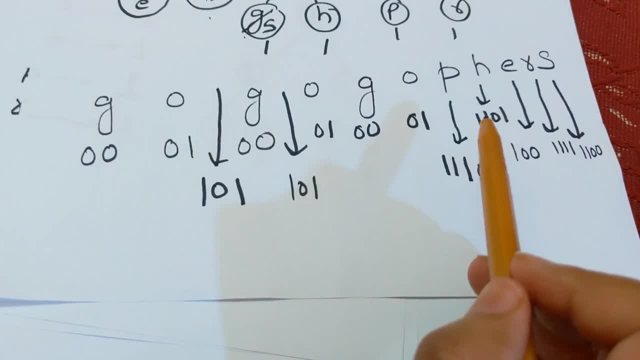 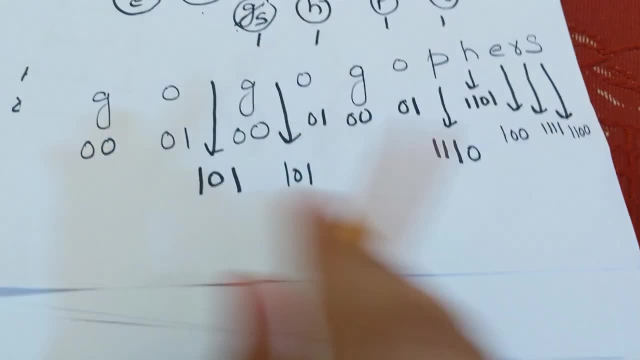 17,, 18,, 19,, 20,, 21,, 22,, 23,, 24,, 25,, 26,, 27,, 28,, 29,, 30,, 31,, 32,, 33,, 34,, 35,, 36,, 37, so that means: 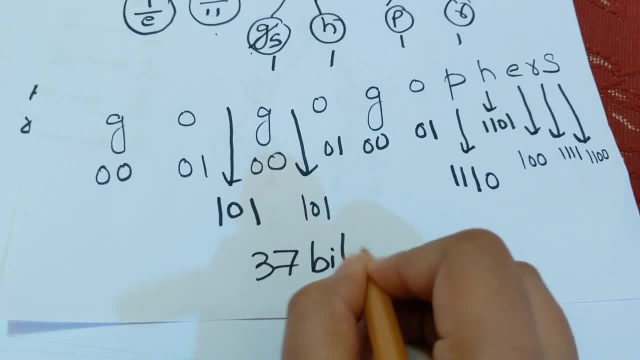 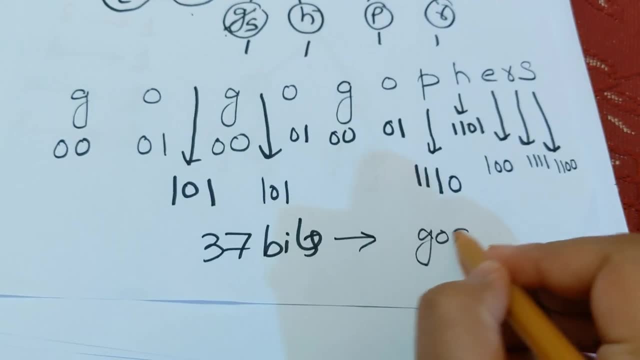 how many bits did you make? 37 bits? how many bits were you making earlier? 104,. now, how many bits did you make? 37? and what is your data information? go, go, go first. so this is your amazing Huffman coding scheme. 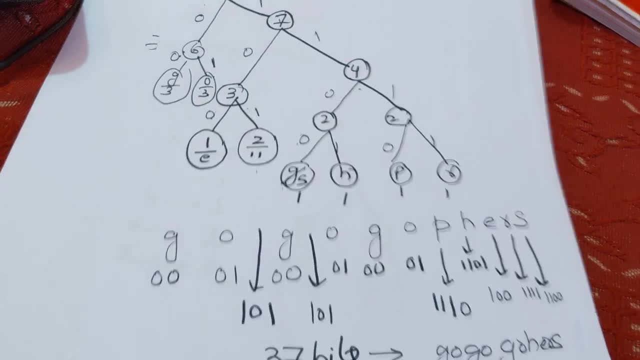 with the help of this tree. I hope you like my video.